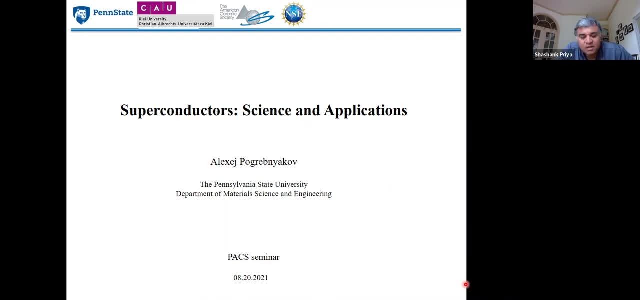 American Ceramic Society, which has provided a great support for our program. And then K stands for Keele, So that the Keele serves as the host university for all the US students which Penn State and American Ceramic Society together select, And these students 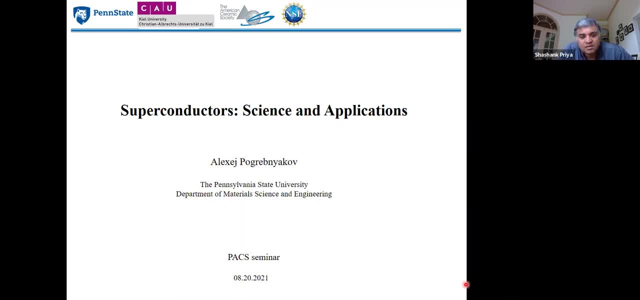 spend three to six months of time at Keele understanding and learning different aspects of smart materials, magnetoelectrics, sensors, biomagnetics- a very diverse range of topics- And this program has been supported by National Science Foundation through OISC, And NSF has really conceived this very creative program to provide. 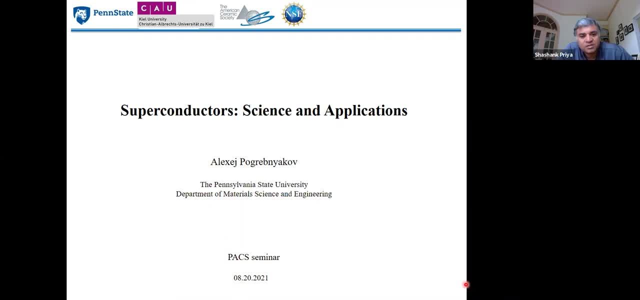 and engage students from all over the world with each other. So our students the first cohort had the chance to spend their time and learn many different things in pin film lab and in magneto ice lab. Our second cohort, because of COVID, has been delayed, But we are hoping that the second cohort can start to. 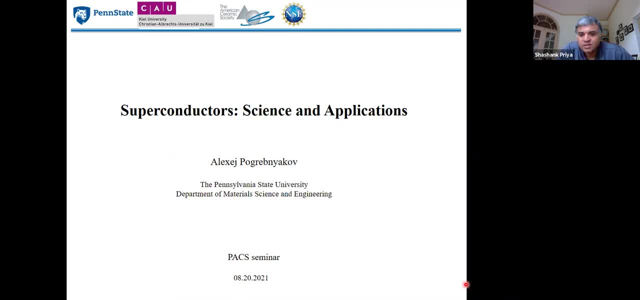 arrive in Keele in early January. So at this point we are collecting actually applications for second cohort and we're making down select And hopefully we'll finalize the list of students in a month or two that they can start to arrange their travels. So if you're a student, a PhD or a master's, 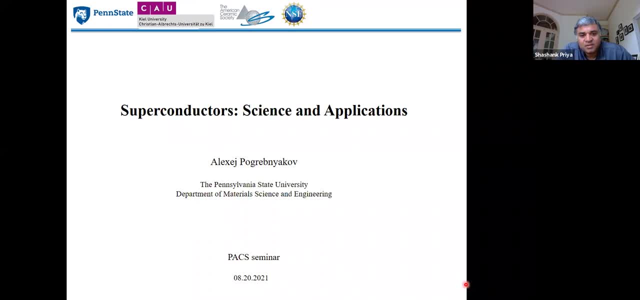 and you are a US person, you're most welcome to apply. Just send your application directly to Sadie Spicer on the call, or you have received email from Sadie and she will get the process started for your application. And so in this PACT program, one of the activities we do is organize these online webinars. 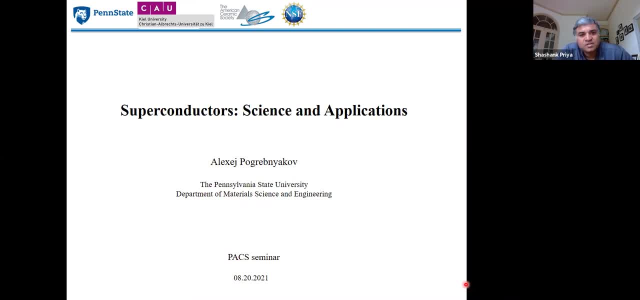 And this is one of the ways we educate our students, both in US and all over the world, And all the great speakers who have come in this PACT seminar. they have provided a very basic tutorial or some background information about a new topic And over the course of the last several months they have learned many different new topics. 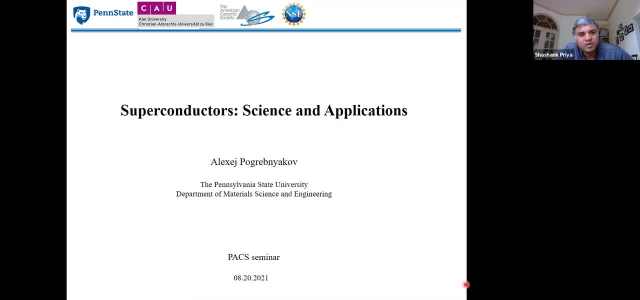 And so today is a very exciting topic of superconductors, which is probably the most famous and popular topic in the world, And we are grateful that Alexei was able to find time and pull together presentation for us And he has a lot of experience in this area. Alex is a very, very 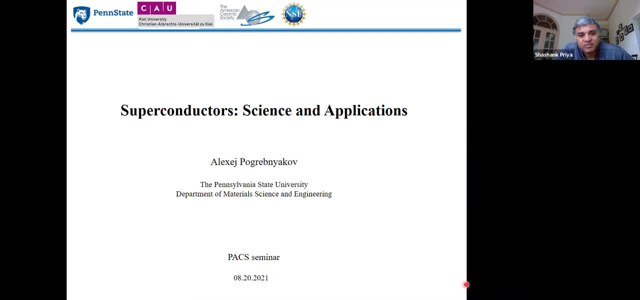 diverse researcher, has done a lot of research in many different domains, like 2D materials and optical materials, And now he's working on acoustics. So he's very well renowned in many different areas And so I'm very thankful Alex was able to find the time to come and give this. 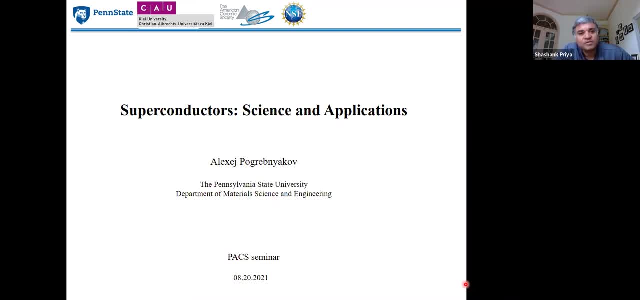 seminar to you And I think you'll learn a lot of new things today in this time. So thank you, Alexei, and I'll pass it on to you. Thank you, Professor Priya, for your introduction, And good morning everyone at Penn State and guten Abend for the attendees of the seminar at Kiel. 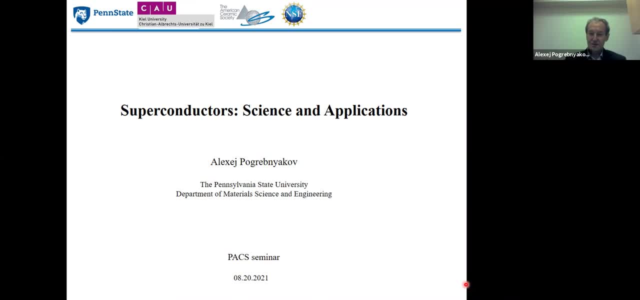 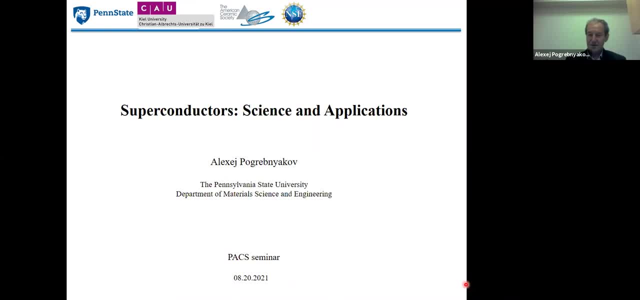 interesting topic. I think it's a very interesting topic. I think it's a very interesting topic And at first glance it would seem that this subject is out of the framework of the Park program, But actually it's not the case, because high-temperature superconductors are in. 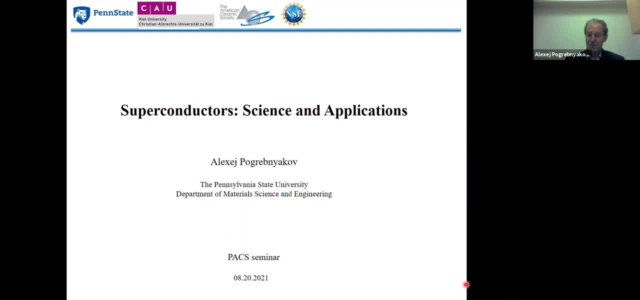 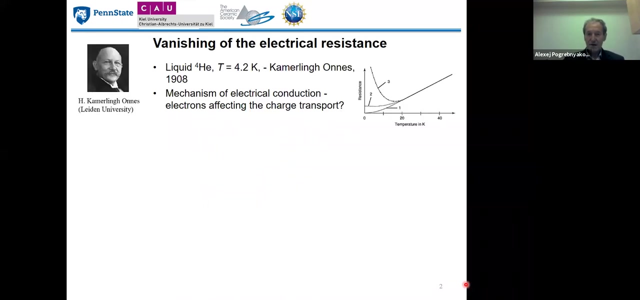 effect ceramic materials and they possess all the properties of regular ceramics, And this affects superconducting properties, as we will see later today. So let's start. and let's start from the beginning, Almost over 100 years ago, at low temperature physics laboratory at Leiden University in 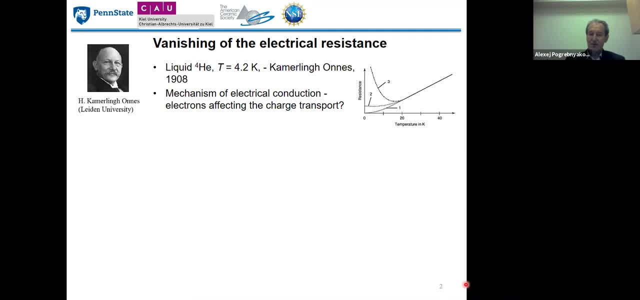 Holland. the director was Kamerlin Onnes, and in 1908 they succeeded in liquefying the last noble gas, helium, and this vastly expanded the areas of research in the low temperature physics, opening the possibility to do research closer to absolute zero. 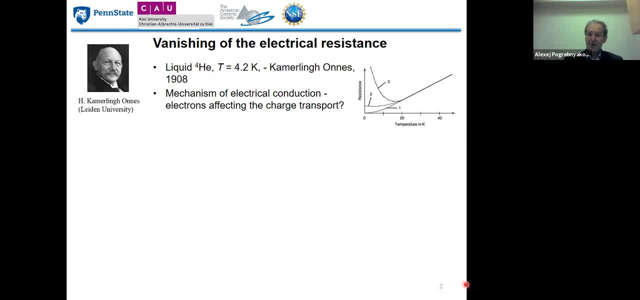 At that time the mechanism of electrical conduction was poorly developed, So there were several ideas, as shown on the plot on the right. For example, James Durer suggested that the lower the temperature, the lower the resistivity would be, and eventually the resistivity will tend to go to zero. 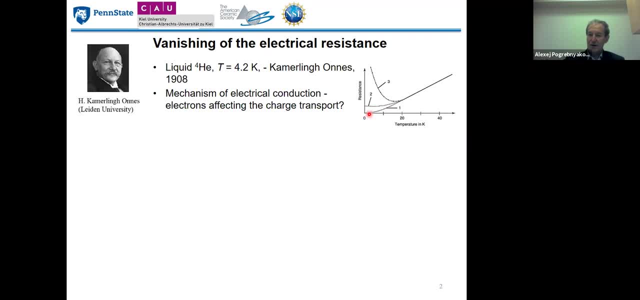 As shown here by the curve number one. It was also known that materials would have some residual resistivity. So at room temperature and slightly below, the resistivity was going linear with decreasing temperature. But then they started and the dependents started to deviate from it. 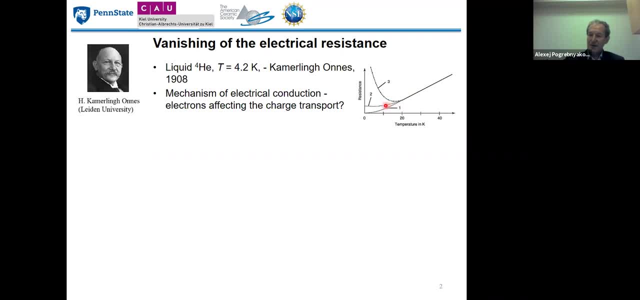 So they could go to zero And so on, deviate from linear dependence, And so the idea was that probably materials would be reaching some residual resistivity. The third proposal came from Thomson, very famous physicist, Lord Kelvin. He suggested that the resistance would go through a minimum. 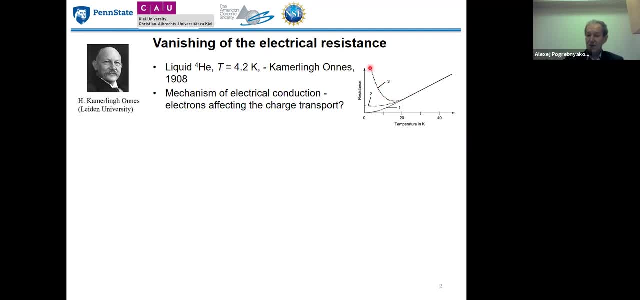 and then would start rising again and the electrons would adhere to corresponding atoms. So Kamerlin and Onnes studied investigations of electrical conduction of pure samples of gold platinum, because the sample at the time could be obtained in pure form. but then he switched over to 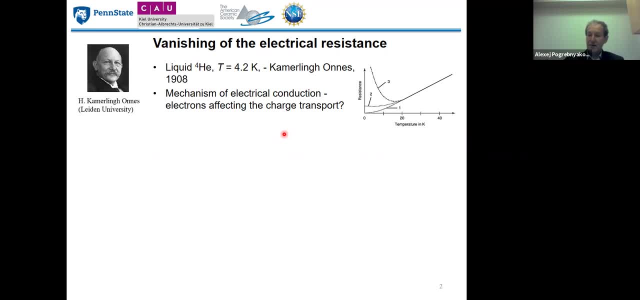 liquid metal, mercury, because after consecutive distillation, that material could be obtained in very pure form. And after some time, what was found? instead of all these predictions, that the resistance of the mercury samples dropped down within a fraction of the degree to a so low value that could not be measurable. 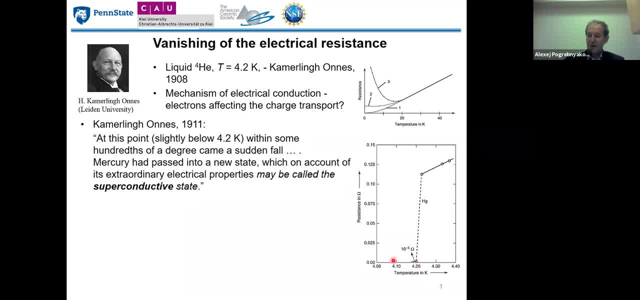 with the apparatus that were available for electrical resistance measurements And, as Kamerlingh Onnes wrote in the proceedings from that institute, that this sample of mercury, this sample, passed through a new unknown state that he called superconductive state. So he himself coined this term superconductive. 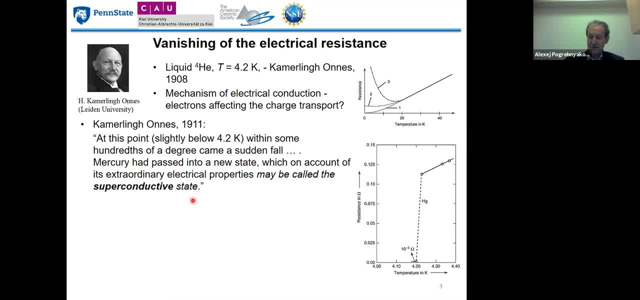 superconductors, superconductivity and so on. So this is one of the main characteristics of superconductors: that at some temperature, which is called critical temperature, the electrical resistance go to the level that cannot be measured. Actually, experiments can be done and were done. 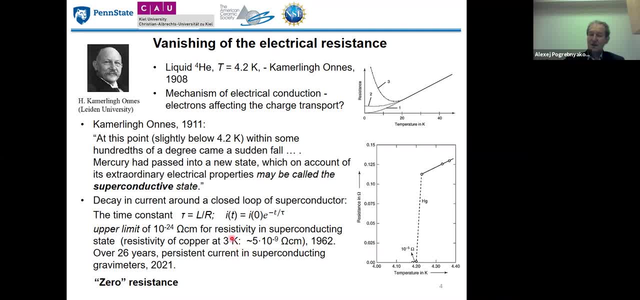 that consisted in inducing a superconducting current in a loop of superconducting sample And the measurements were done over the decay of the current with time, as shown by this equation, And, for example, in 1962, after two years of this studies. 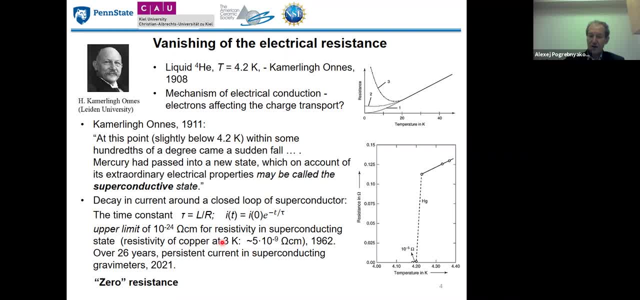 it was found that the upper limit for resistivity of superconducting state was 10 to minus 24 ohm per centimeter. For comparison, at the same temperature of 3 Kelvin the resistivity of copper is 5 times 10 to minus 9 ohm per centimeter. 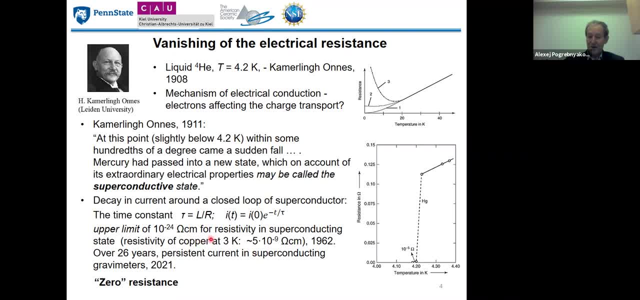 So the difference between this conductivity of superconductor and copper is similar as the difference between the conductivity of metals and insulators. And recent data in Belgium. they were conducting gravimetric studies using superconducting gravimeters and the persistent current as of today, July 2021,. 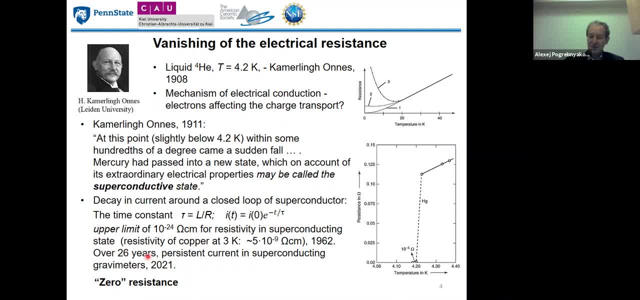 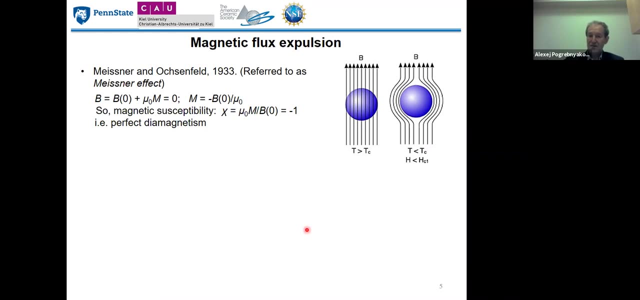 persisted for over 25, 26 years. So this is one of the main properties of superconductors. The next very important property of superconductors is magnetic flux expulsion. It was discovered by Meissner and Ochsenfeld in 1933,. 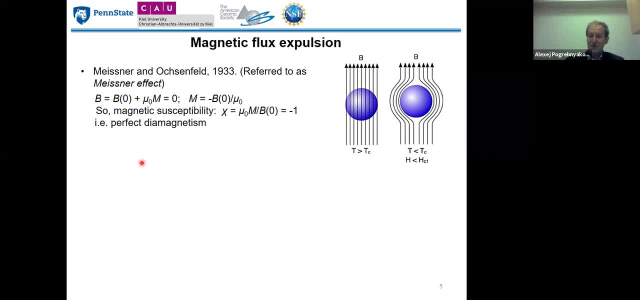 and currently it is referred to as Meissner effect. It turns out that um if we place a superconducting material into a magnetic field, then at temperatures that is higher than the critical temperature, then this material is in normal state. 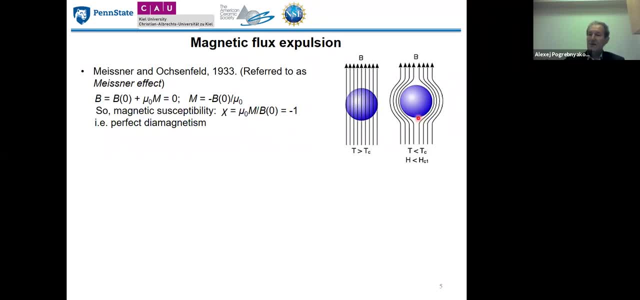 then, if we just decrease the temperature, the magnetic flux will be expelled, expelled from the interior of the sample. This is a Meissner effect, So superconductors behave as a perfect diamagnetics. Magnetic susceptibility equals to minus one. 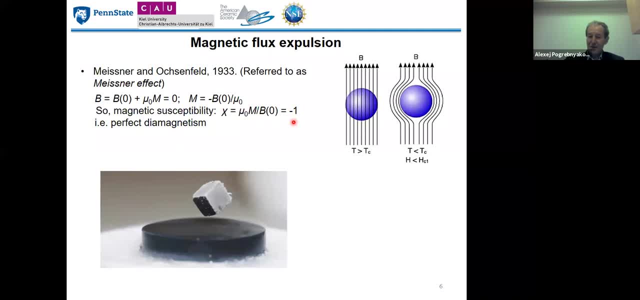 This brings about a very interesting um um effect as magnetic levitation. If one places a sample of ferromagnet over the superconducting material that is in superconducting state, as shown here, it will float over the surface of superconductor. 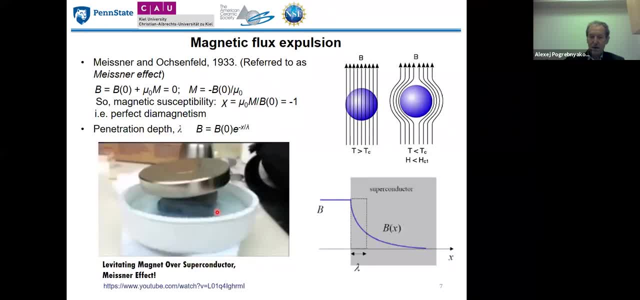 And um, let's, um, um, let's watch some video. If you are lucky, it will work. So what you see here is a rotating ferromagnet sample of the high temperature superconductor that is placed in the center of the circle. 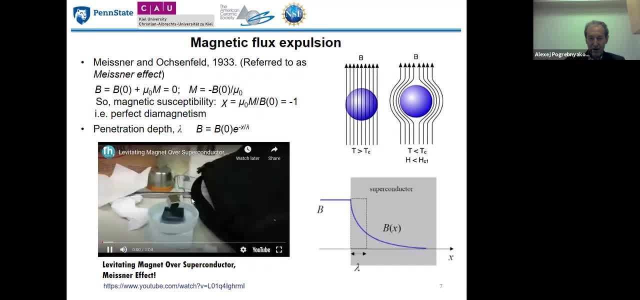 Now you can see that it is. uh, it is a magnet. it is a magnet and it is using the magnetic flux of the magnet. And when we look at the bottom of the circle, we see that it is rotating, uh. 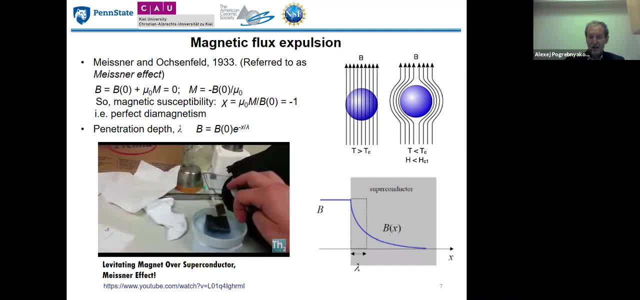 uh uh it is a magnet. And uh, it is a magnet that is uh uh rotating, uh uh temperature superconductor that is placed in the liquid nitrogen and it is. its temperature is below superconducting. 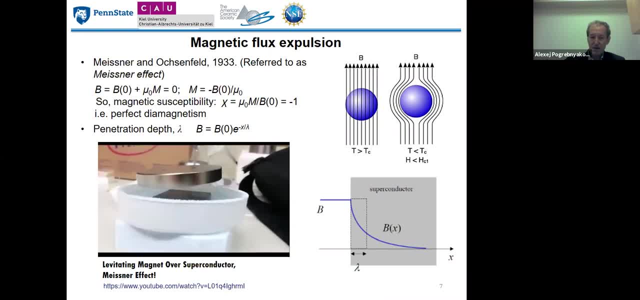 transition temperature, so it's in the superconducting state. this is another example. so what happens actually is that magnetic flux is zero in in the interior of the sample, but magnetic field penetrates into the surface of superconductor and the, according to this expression, it's. 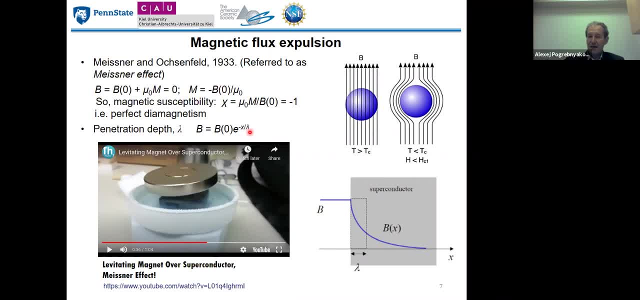 exponential dependence and the length constant is called penetration depth. um marks here is lambda and so at this surface layers there is a current, normal current that creates magnetic field. that exactly cancels the magnetic field from the external source and that's how the magnetic field inside the sample 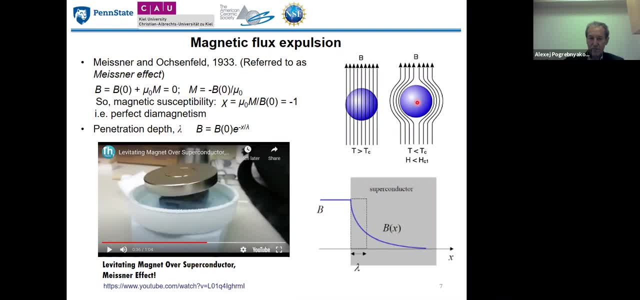 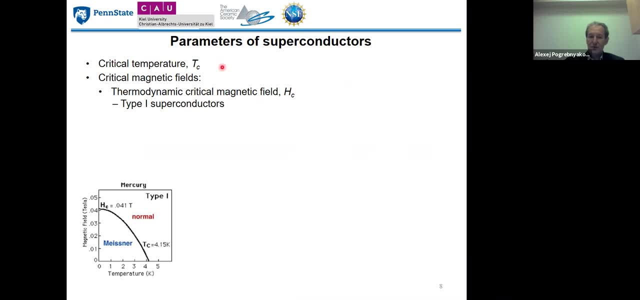 becomes zero. so parameters of superconductors: first of all, we already see so that that was a critical temperature. then there's critical magnetic fields. there are several critical magnetic fields. uh, first of all it's a thermodynamic critical magnetic field. uh, it's a characteristic for type one. 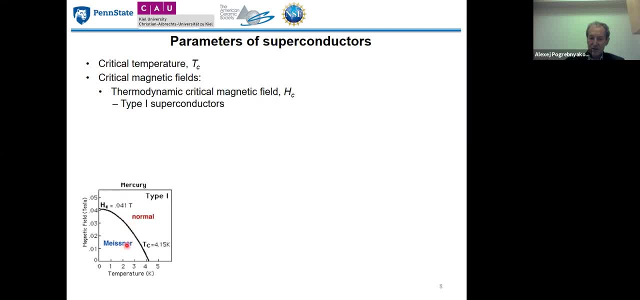 superconductors. so superconductors can be either in meissner state, where there is no magnetic field, or if the external field is over, exceeds the critical magnetic field, the, the superconductor goes over to the normal state and of course, this thermodynamic critical temperature. 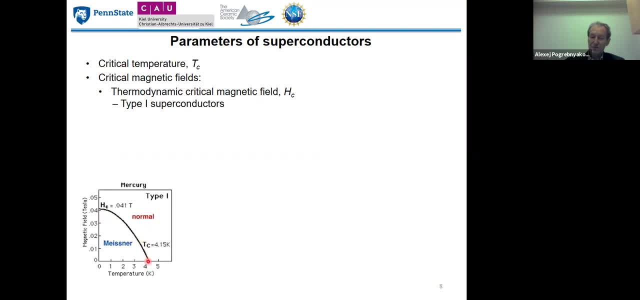 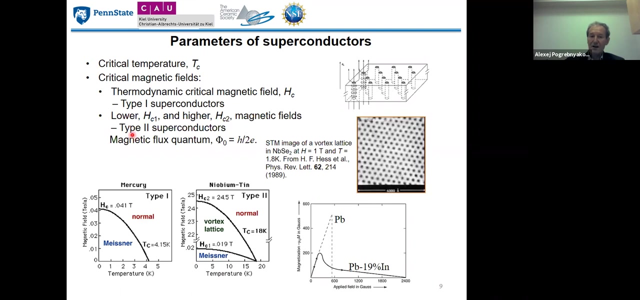 depends on temperature and it becomes zero at critical temperature of a particular superconductor. so this plot shows the dependence of thermodynamic critical field. for mercury that has a critical temperature of 4.15 kilo. so there is another type of superconductors and most of the superconductors are 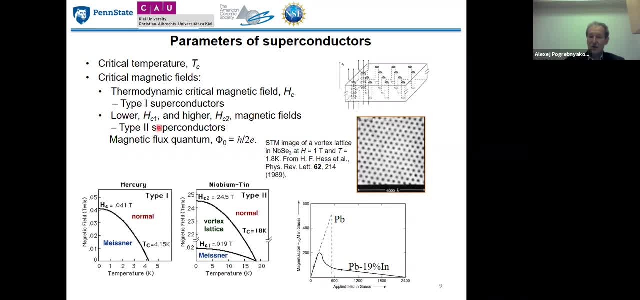 type 2 superconductors. they have two magnetic critical fields- lower critical field and the higher critical magnetic field- and the phase diagram is as follows: for relatively low external magnetic fields the sample is in meissner state, so no penetration of magnetic field magnetic flux into the interior of the 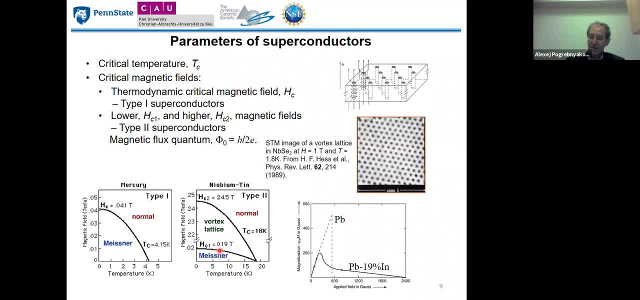 sample. but if the external magnetic field exceeds the lower critical field of a sample at a particular temperature, the magnetic flux starts to penetrate into the sample and it penetrates its as a vortex lattice, as shown here, shown here on this cartoon and the here is the top view of 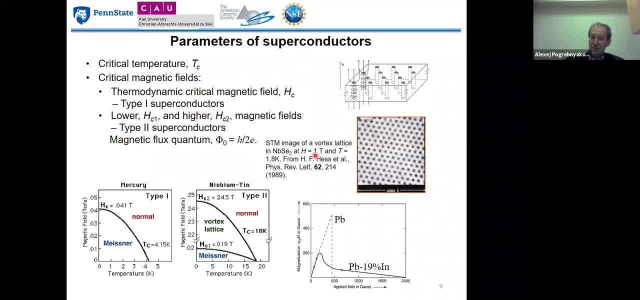 scanning tunneling magnetometer. this is the scale bar is 6000 angstroms. so we see this is a perfect, ordered lattice of magnetic flux vortices that penetrate into the sample. within this vortices the sample is in normal state and outside the 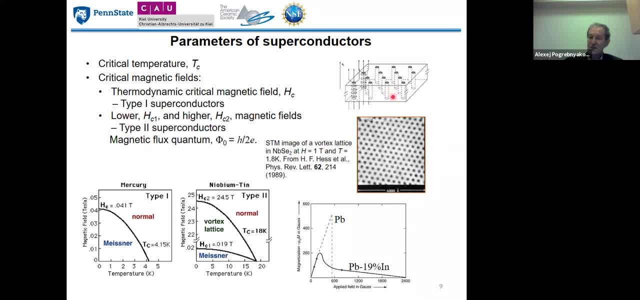 vortices. between the vortices it's still in superconducting state and only the external. after external magnetic field exceeding the upper critical field, the sample becomes fully normal. no superconductivity and for example, this plot shows that lead, pure lead, is a type one superconductor. 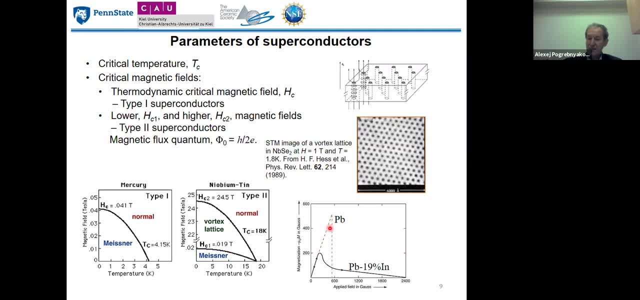 is shown here by dashed line. it has thermodynamic, particular thermodynamic critical field that is below 600 gauss. but the lead allied with indium is a type two superconductor and here we see that this peak corresponds to lower critical and here we see that this peak corresponds. 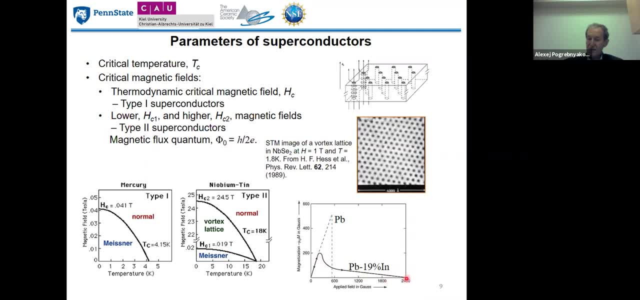 to lower critical field and this value of about 2400 gauss is an upper critical field for lead indium. this magnetic flux quanta contain a quantum of magnetic flux which is shown in this expression: h is a plan constant and e is a electric charge. electronic electric charge of the. 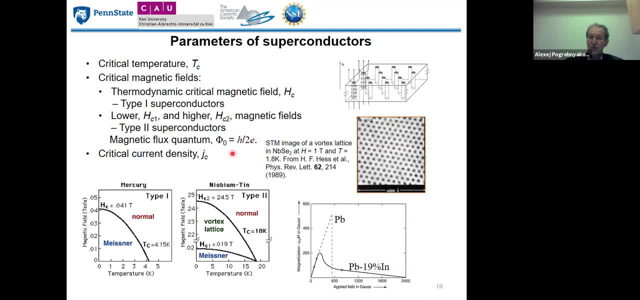 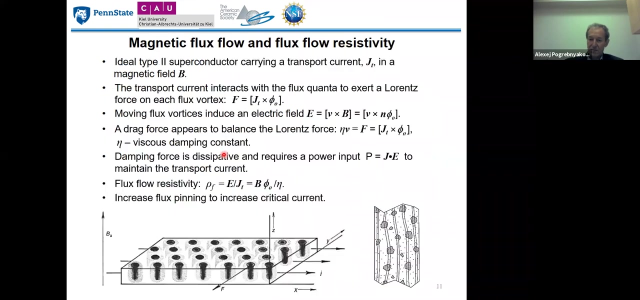 electric. and one more parameter of superconductors is critical current density. so superconductors can carry a current but if the current strength or critical current density exceeds some critical current density, exceeds some critical value, superconductor goes over to the normal state. and if we pass a current 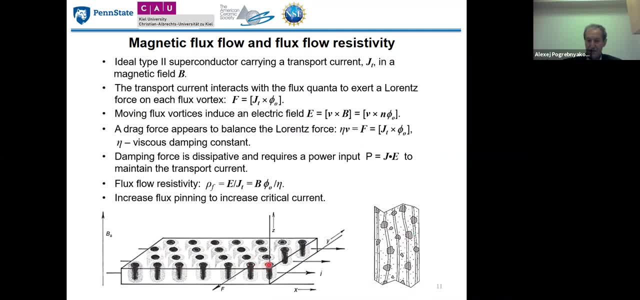 along x direction, as shown on this on this carton, and turn on the external magnetic field normal to the current direction. then in pure and very ordered samples the vortices start to move and the movement is caused by lawrence force and this movement will bring about. 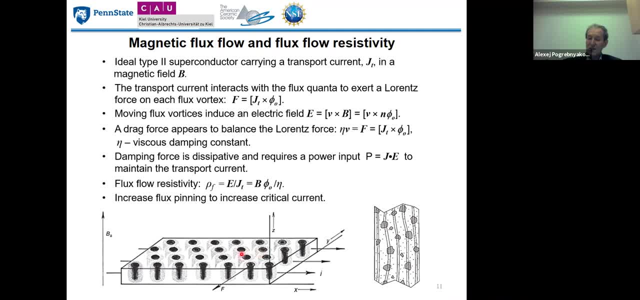 dissipation. so although the sample will be in superconducting state, this current will dissipate and there won't be persistent current in the in the superconducting samples, although it is in superconducting state. so this phenomenon is described by flux flow resistivity, as shown in this. 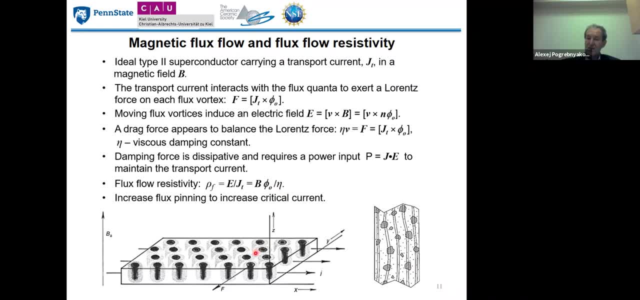 expression. so to prevent, to suppress the dissipation, to make the current flow without resistivity, as in resistance, as in this should be in superconductors. we have to prevent this vortices from moving. it is made by introducing making the samples dirty. this is jargon in 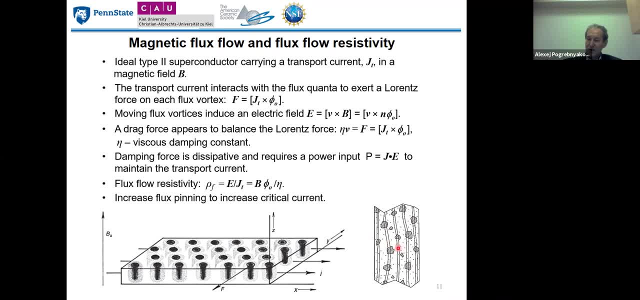 superconductor community. so making the samples duty can be achieved by alloying or adding some particles or irradiating, creating defects, structural defects, polycrystalline samples. grain boundaries of of the samples will act as pinion sites, so vortices will be. 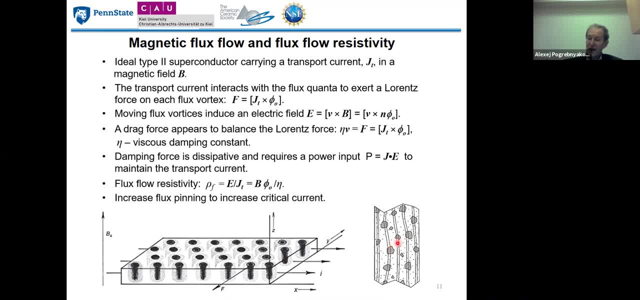 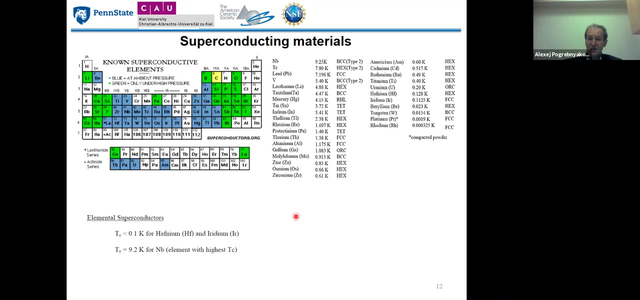 attracted to to these centers and unless the current is so strong the the vortices will tear of this pinion sites. there will be no movement of vortices and the current will flow without the resistance, so superconducting materials. here we see the periodic table and blue. 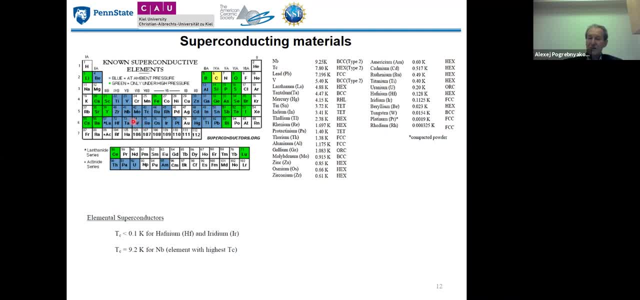 color marks the elemental superconductors, that are superconductors at ambient pressure. and here we see that. here we see just examples of some elemental materials with corresponding critical temperatures. so the maximum critical temperature of elemental material is 900.25 kelvin for niobium. 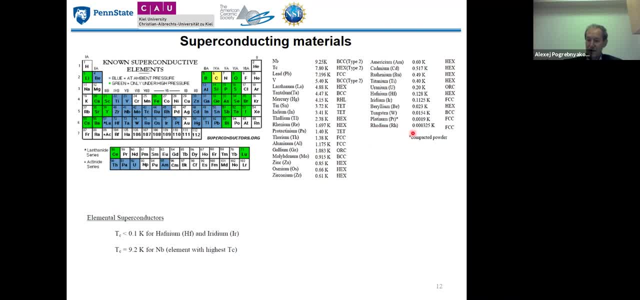 and there are samples with very small elements with very small critical, very low critical temperature. by green color mark the elements that become superconducting at higher pressure. so these are elemental superconductors. but there are a lot of superconducting alloys, for example, there are many. 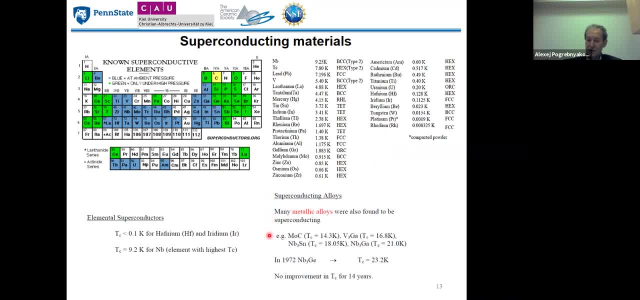 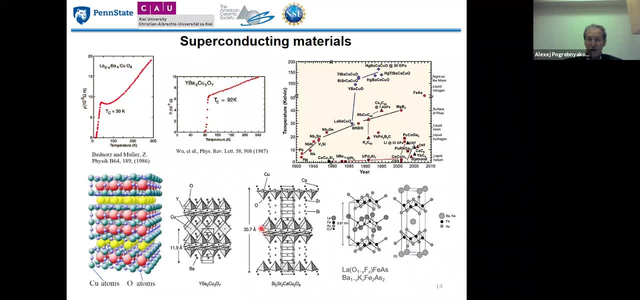 metallic alloys and many of them are used in applications. so we continue on superconducting materials, materials, and here we see that in 1986 there was discovered, there was discovery of high temperature superconductivity in, of high temperature superconductivity in this complex of oxide: lanthanum, barium. 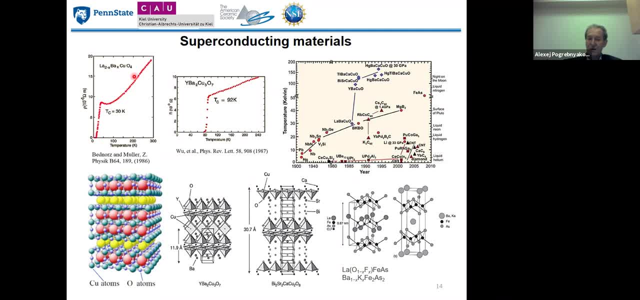 this complex of oxide: lanthanum, barium copper oxide. just after several months after this discovery, the critical temperature was raised, raised from 30 to 92 raised, raised from 30 to 92 kelvin in the etrium barium copper oxide. after that, during this, 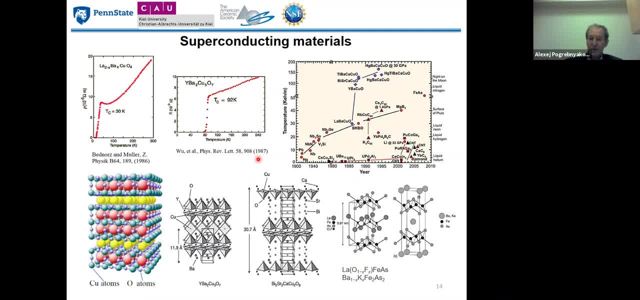 time after this discovery. time after this discovery, the critical there were the critical: there were discovered multiple high temperature superconductors of this family and other families of superconductors of this family and other families of superconductors for, for example, high critical temperature, for example. 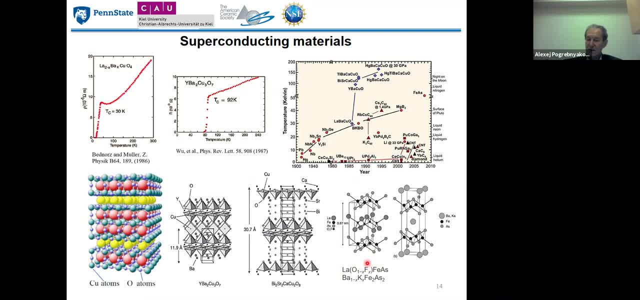 superconductors that contain iron. iron, that was that was considered a no-go in the superconductivity, superconductivity research. it was considered the iron was because it's it has, it's because of it has ferromagnetic properties. it was the magnetic field suppresses the superconductivity. 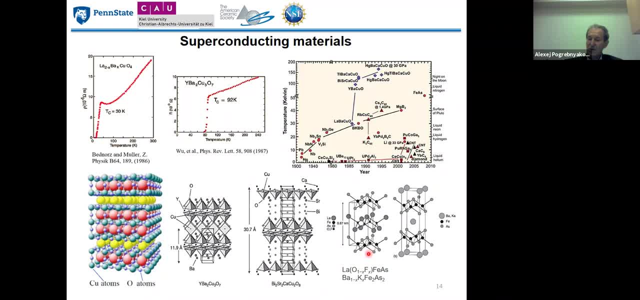 it was thought that no way that samples containing iron would have appreciable value of critical temperature. turned out that that was not right, and these materials have critical temperatures of about 55 degrees kelvin. so what we see is that here this colored cartoon shows the atomic distribution in e3, barium copper oxide. 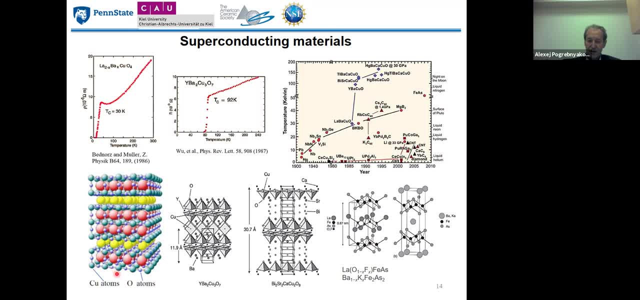 and copper atoms are shown here and oxygen atoms are shown here and red spheres stand for barium and this yellow, green spheres stand for etium atoms. the conductivity, or superconductivity, occurs within this copper oxide planes, so these samples are highly have highly anisotropic, anisotropic properties. 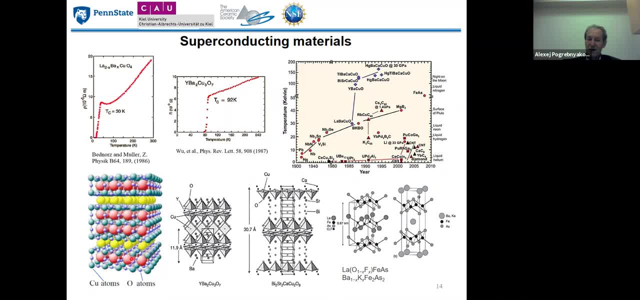 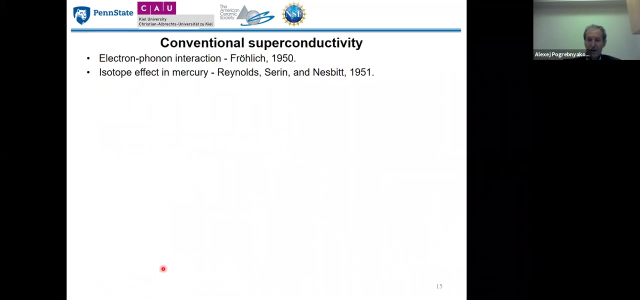 conductivity within these planes are much higher than conductivity in the normal direction. so this is typical ceramic superconductors, uh, the brittle um, and we'll see how it affects the properties of, in particular, current carrying capabilities of these materials when we go to discuss the applications. so, um, conventional superconductivity, um. 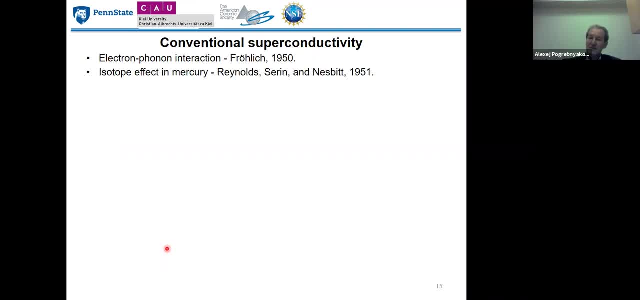 Superconductivity. after the discovery of superconductivity and up until 1957, the mechanism of superconductivity was not understood, despite the many brilliant minds that tried to tackle this problem in particular- So many. I won't dwell on it. 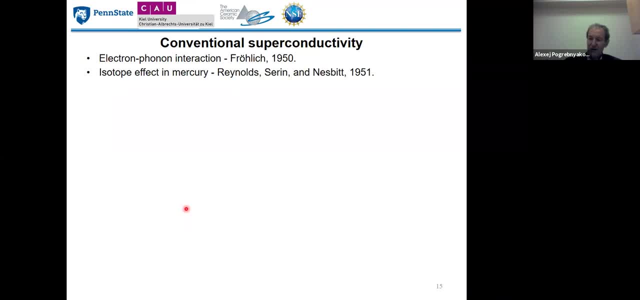 many researchers, very famous theorists, tried to solve this problem. They could not succeed. So the first indication come from a theory considering interaction of electrons with phonons in solid state. So Froelich in 1950 theoretically described this electron-phonon interaction. 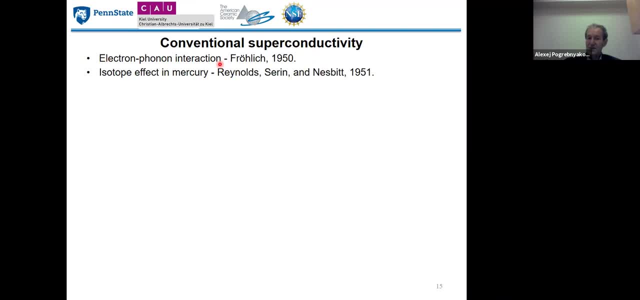 In particular, electron-phonon interaction brings about the resistance of the samples. The stronger electron-phonon interaction, the higher the resistance of the sample The next year. it was found that mercury has isotope effect. So when adding atoms with the same atomic number, 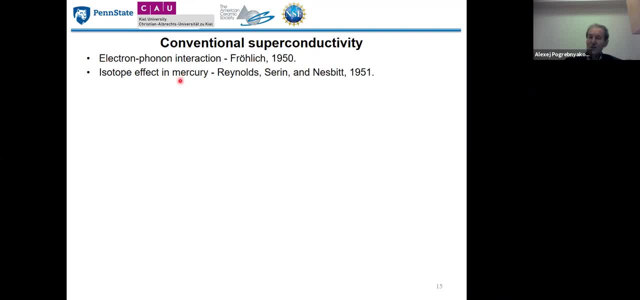 so the same chemical element, mercury, but the atoms of different atomic weights would change the critical temperature of the mercury, which meant that somehow the lattice- iron lattice- is involved in the superconductivity phenomenon, And in 1956, Cooper showed that. 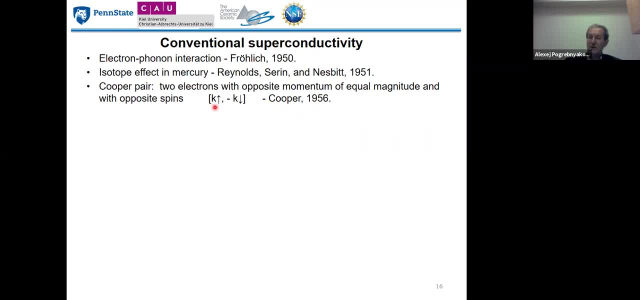 again theoretically, that the electrons with opposite momentum and opposite spins would have a strong correlation And this correlation would depend upon the interaction between these electrons. Any attractive interaction between the electrons, however small, would bring about the would brought about the correlation. 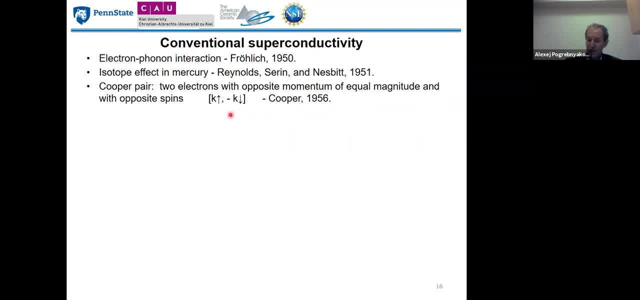 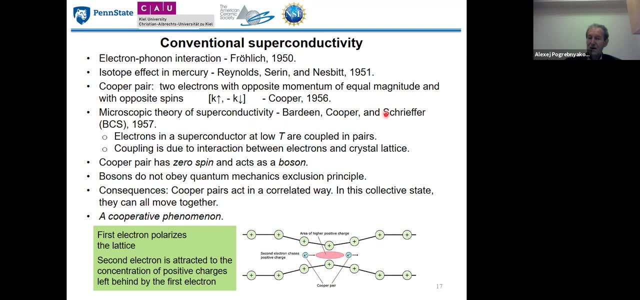 between these pairs of electrons. And in next year Bardeen, Cooper and Schrieffer produced eventually the first successful theory of microscopic theory of superconductivity based on this property of Cooper instability and Cooper pairs. So in this theory 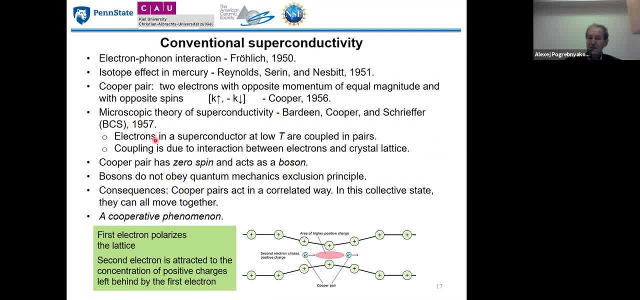 which is referred to as BCS theory. electrons in a superconductor at low temperatures are coupled in pairs, And coupling is due to interaction between electrons and crystal lattice. So since normally, electrons being fermions, cannot occupy the same quantum mechanical states, 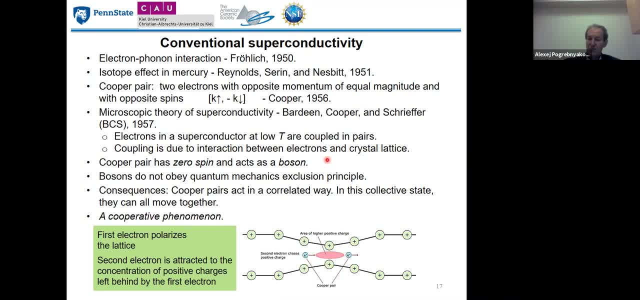 and they will be repelled from each other strongly by the Coulomb forces. But when they form Cooper pairs, then this composite, courageous Cooper pairs will have zero spin And then they will act as bosons, And bosons are quite different from fermions. 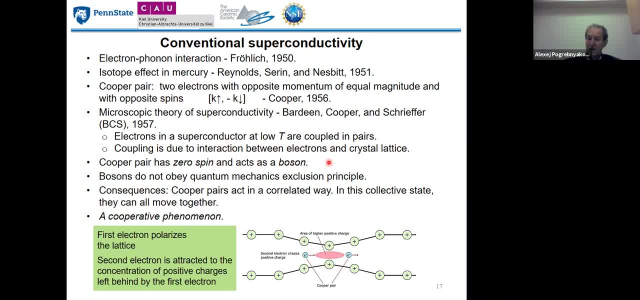 because they kind of provide the same quantum mechanical state as we can, as it all known, in lasers, for example. that's photons can go into the same emitted photons. photons go into the same state. That is why laser radiation is coherent And this: they have all the photons. 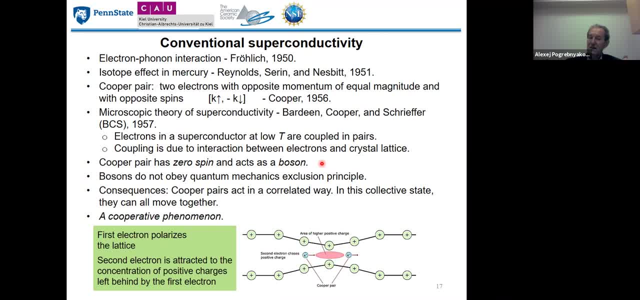 the more the number of photons, the more readily they condense in one particular quantum state. So that is why the laser radiation is monochromatic, is one color, And so this is a property of bosons. So again, the bosons, unlike fermions. 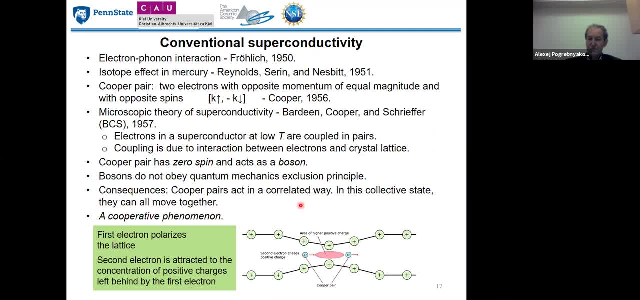 do not obey quantum mechanical exclusion principle. As a consequence, the Cooper-Payer Act pairs in a correlated way. So this is a collective state and they, similar to photons, they could move all together. So this is a cooperative phenomenon, A very, very 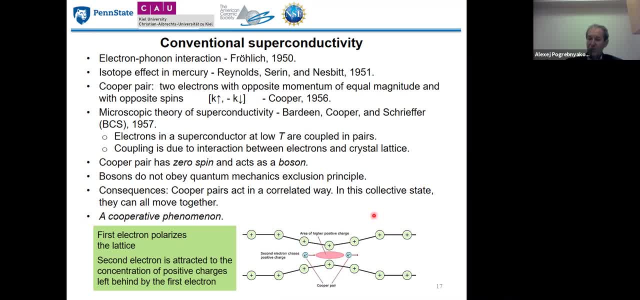 crude way to imagine why electrons in a lattice from Cooper-Payer's would be. just consider one electron that moves along this ordered rows of electrons, And this electron would attract this ions, And so it polarizes the lattice. Next electron that would move after this: 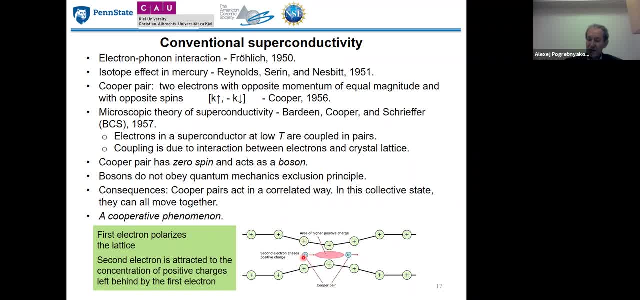 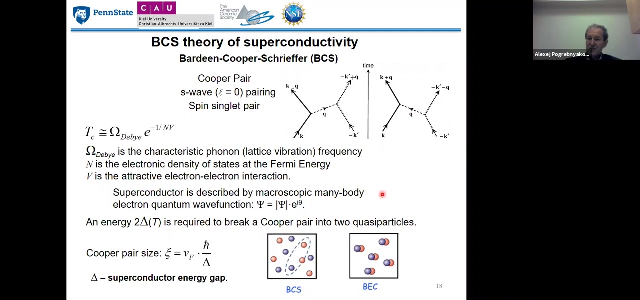 would feel that there's an increased positive charge, and so that's how this electron- second electron- would be attracted to the first electron, while this lattice polarization. that's how this picture of superconductivity works. So this is where this happening occurs. So the thing is. 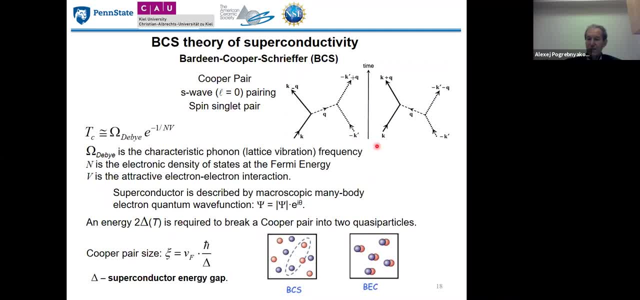 it's the same principle that we used to do in quantum, quantum theory and actually, if you want to, you can look at the building block. actually it was a building block, but it is a building block, but you're not going to be able to do two building blocks. 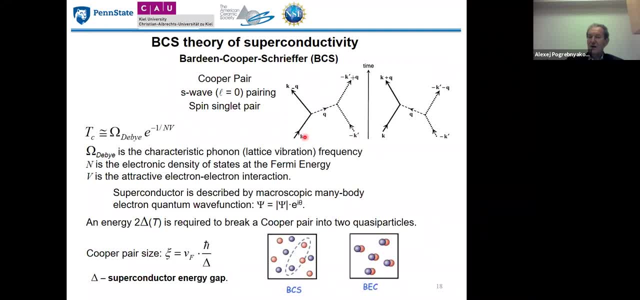 with two building blocks because they're different. So you can see the whole thing in the northern part and the northern part, but it's equally optimal And even if the building blocks- the building blocks that were placed in the southern part- are like this: 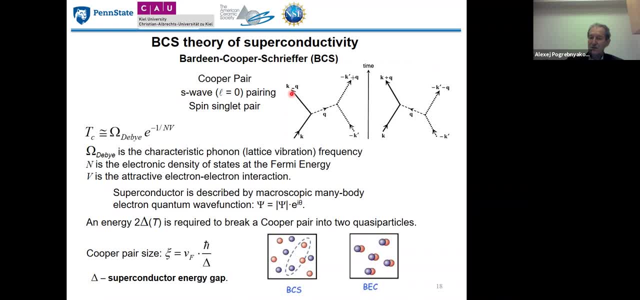 they're not going to move any further. So instead q momentum, the next electron, absorbs this phonon and this scattering. so this scattering process brings about this correlation between these two electrons As a critical temperature was obtained in this BCS theory, you can see that this is 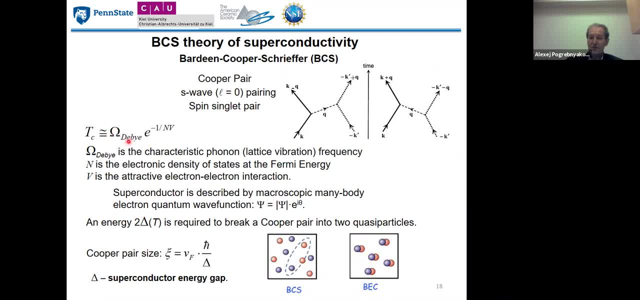 some characteristic frequency of a material, in particular Debye frequency. and here we see that in the exponent there's electronic density of states at family level and V stands for attractive electron-electron interaction and the interaction comes from Friolich-electron. 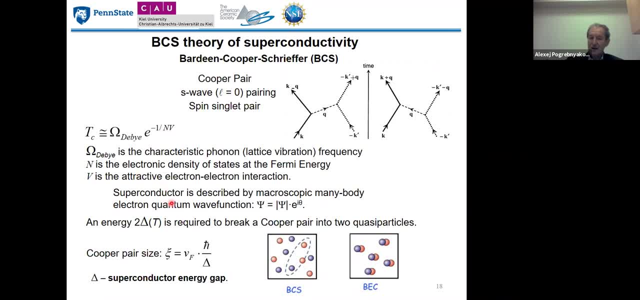 phonon interaction. So superconductor is described by microscopic, macroscopic, many-body quantum wave function, and to break the Cooper pair into particles one has to apply an energy to delta and the Cooper pair size or coherence length, xi, shown here. 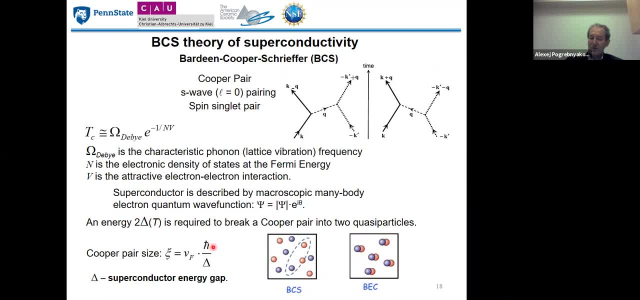 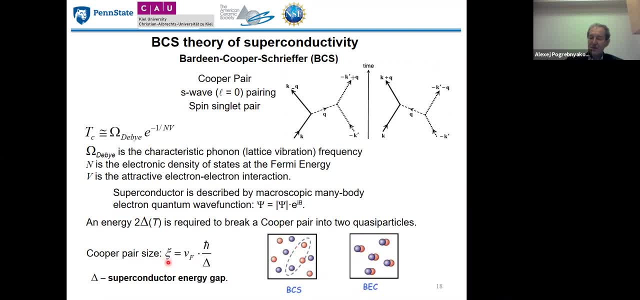 For BCA superconductors, this coherence length is very large compared to the distances between the conducting electrons, So there is a lot Docker pairs that are interpenetrating into each other. So this is the correlation. That is why this superconducting state is so stable. It iscially closely, closest to nectar hierarchy. So that's the reason that with the drug we are able to calculate superconduct, So you can even just conjugate this superconducting state and sink or respond to the organic electrons. 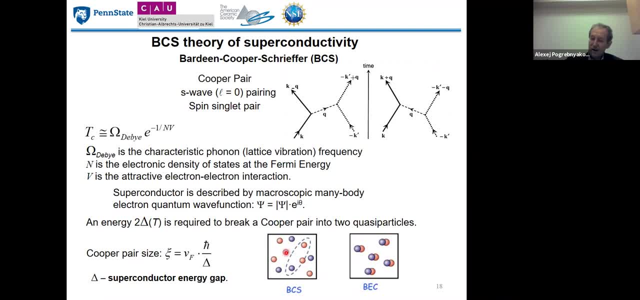 So there's not a Mason-hyperconducting glaze. So there is not a Mason-hyperconducting glaze. it's difficult to break a single particular Cooper pair because they're all interconnected correlations Currently. so this theory, BCS theory, 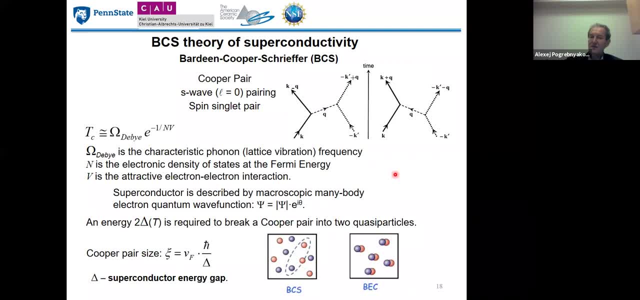 was developed further in several years after the publication, and the theory of superconductivity was the most accurate physical theory in condensed metaphysics. So high temperature superconductors that were discovered already over 30 years ago have much stronger interaction between the electrons. 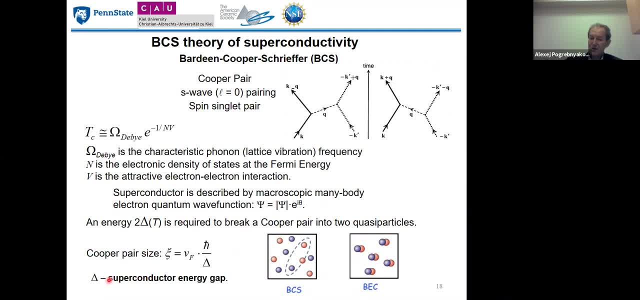 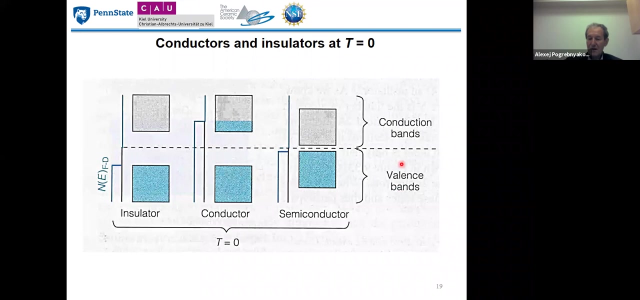 and this superconducting energy gap is much larger. So the Cooper pair size is much smaller, as shown on this cartoon, And up to now there's no theory- accepted theory- of superconductivity in high temperature superconductors. So let's see. 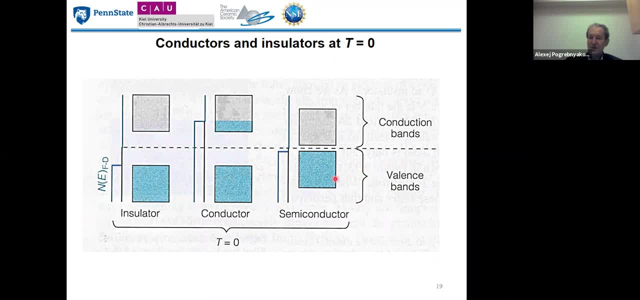 How this superconducting energy gap where it opens. So here we see energy band diagrams of various materials, insulators, conductors and semiconductors. And in insulators we see that the valence band is fully occupied and the conduction band is fully. 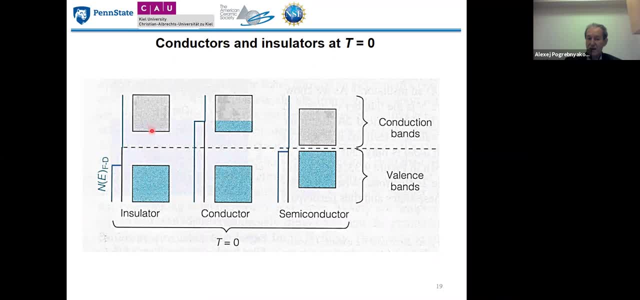 unoccupied, So there is no conducting electrons There's, so the insulators are insulating In conductors. there is some number of occupied states in the conduction band but other states are unoccupied. So when we applied the voltage 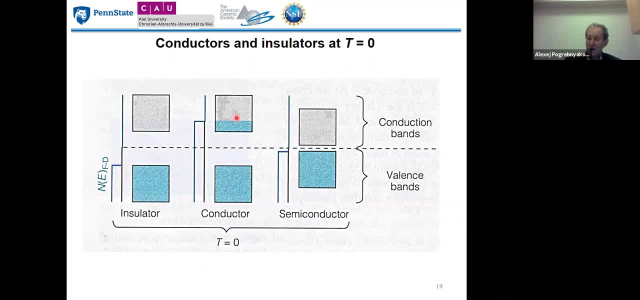 the electrons can go over to other empty states, and that's how the current can be can be transmitted by a conducting. materials in metals And semiconductors are similar to insulators, but the band gap is much smaller than in insulators. 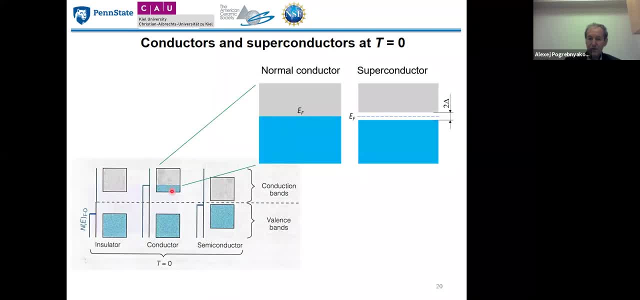 So if you look at the metals, so normal conductor, so electrons occupy energy levels in the conduction band up to maximum, some maximum energy which is called Fermi energy. And when in superconductors the gap arises between the occupied states, 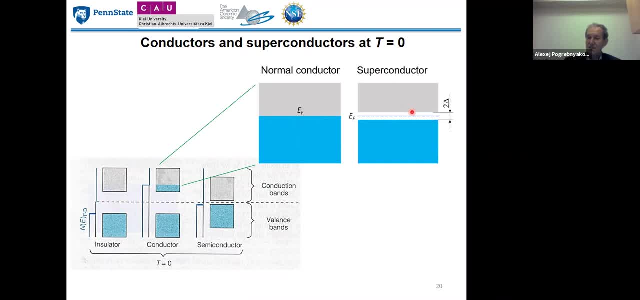 and unoccupied states And this gap near the Fermi surface or around the Fermi surface, this gap is equal, equals to two delta, two superconducting gaps. This value of superconducting gap actually can be measured, directly measured. 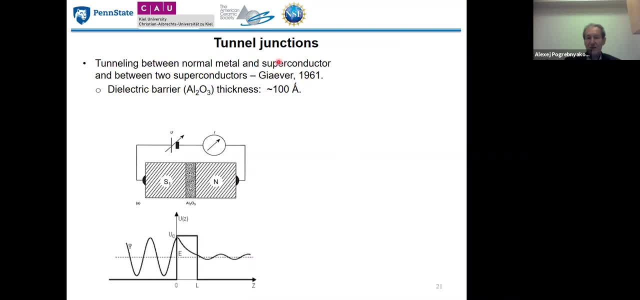 In 1961, Gehrle conducted experiments and he was passing current between the normal metal and the superconductor, And this thin films were separated by dielectric barrier, alumina in particular. So he started he deposited aluminum films on glass substrates, oxidized aluminum. 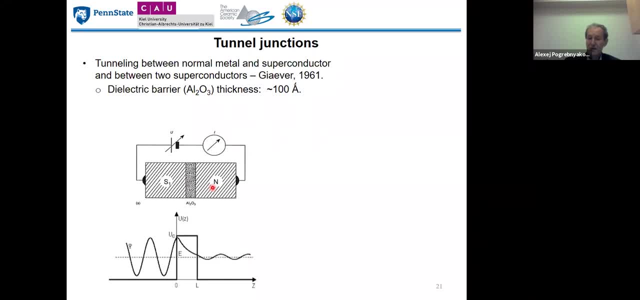 and it deposited on top of this material other films. so, and what was found? that the current was not passing up until some value of applied voltage, and this value equal, equals exactly of superconducting energy gap in a superconductor that forms this junction and three minutes. 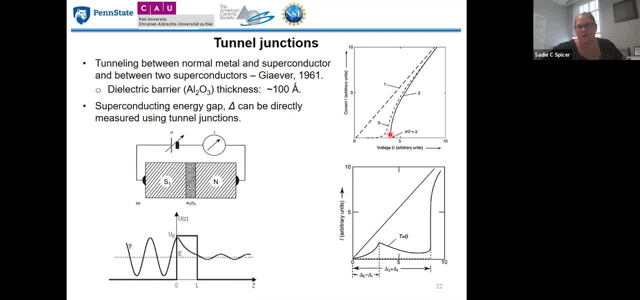 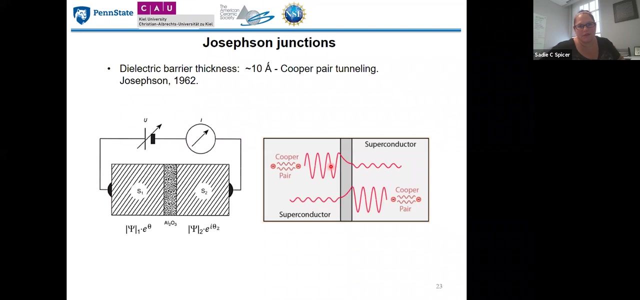 yes, again three minutes, so we have time for questions. please, wasn't it 45 minutes? yeah, if you, if that's all you have left, um, we can finish it. i just wanted to make sure there was some time at the end for questions. you can continue. um, if we decrease the barrier thickness to tenor astrons, we would have 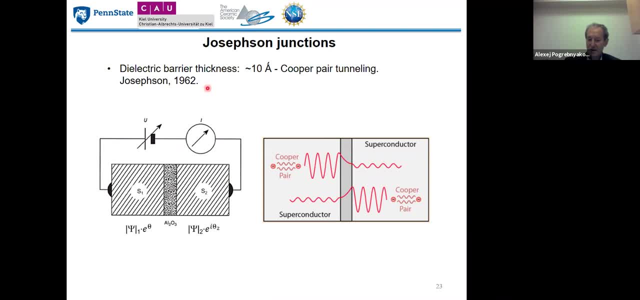 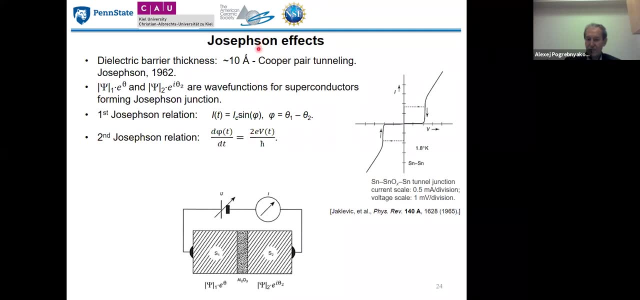 cooper pairs tunneling that was predicted theoretically by josephson in 1962 and this. there are two types of josephson effects that occur in this type of junctions: constant current josephson effect and the alternating current current josephson effect. these effects are widely used in applications. 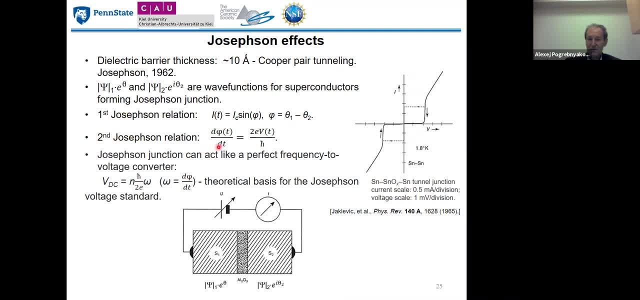 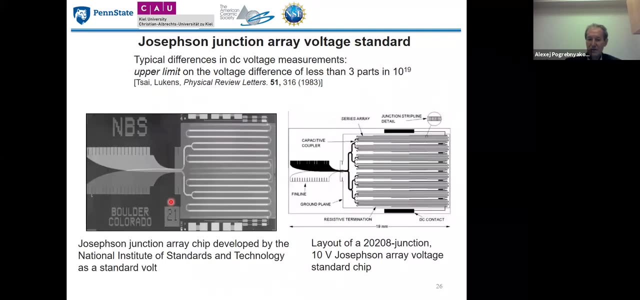 for example, this second josephson effect is used in um frequency to voltage converters and used in voltage standards. and here we go over to the applications. here we see that the josephson junction areas are used in standard of volt, for example. this is the same layout. this is a 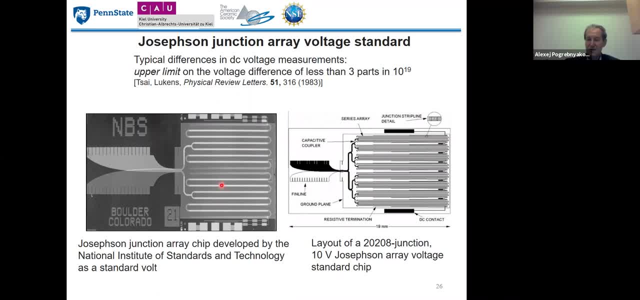 um, you can see that the josephson junction area is showing a same s? m image of a layout of 20 208 208 junctions for 10 volt. uh josephson uh area voltage standard tip. uh. that's because, every particular, why such a large number of junctions? because the voltage drop. 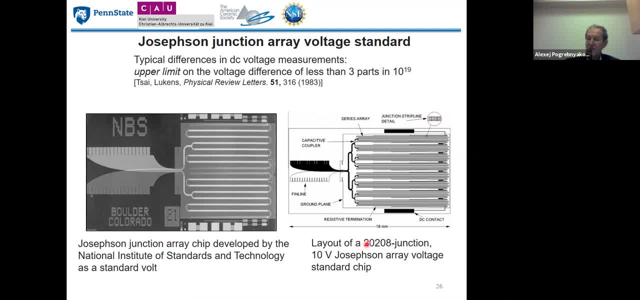 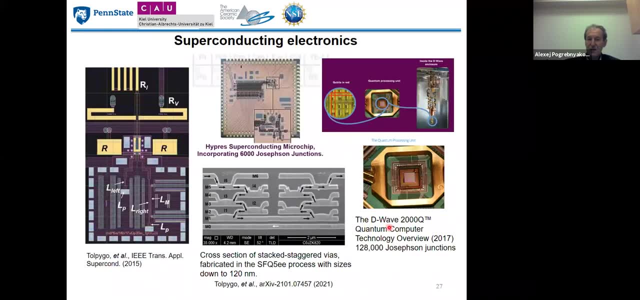 on each particular junction is very small. so to get the 10 volts um drop we use the same idea. you have to have areas of the junctions. So superconducting electronics is based on Josephson junctions. Here you see examples of micro-circuits. 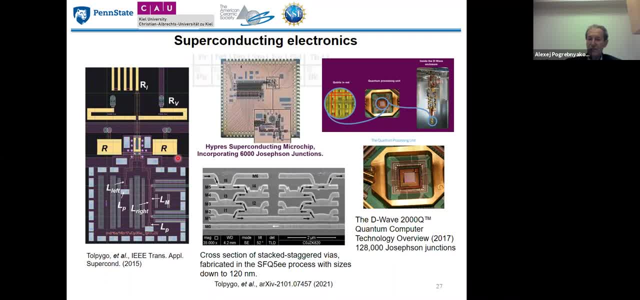 superconducting micro-circuits and they are made of various numbers of Josephson junctions. This is a cross-section of superconducting circuits, So there's a multi-layer structure that contains junctions in different layers. So this Josephson junctions are used. 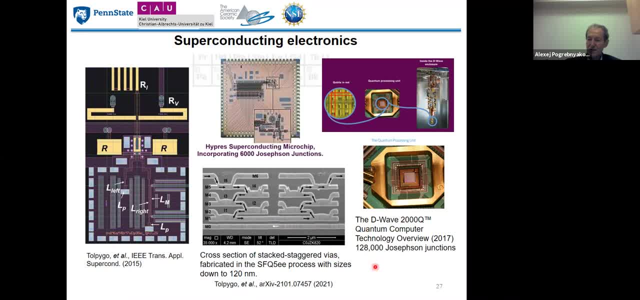 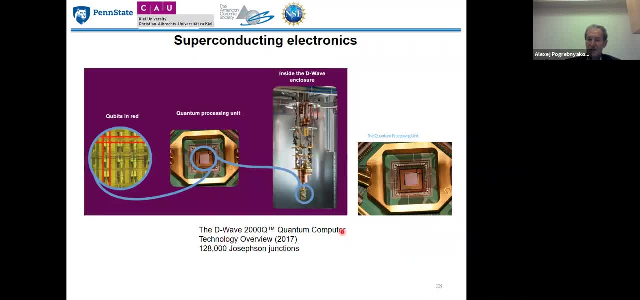 in high-speed electronics and in particular in superconducting supercomputers. It's shown here for the DeWave company This is a working quantum computer that contains 128,000 junctions. So these are applications of superconductors in electronics. 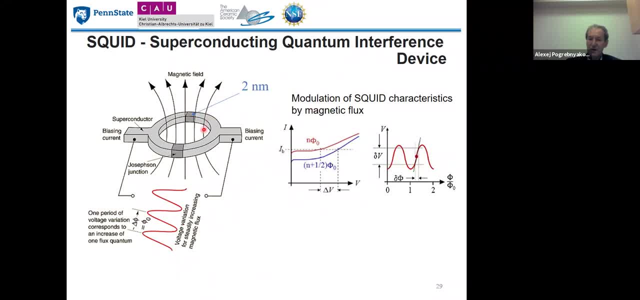 single Josephson junctions. Now, if you put this Josephson junctions in a superconducting loop and apply, pass the current through this loop, the current will split between these shoulders and go into and then combine into this left electrode. 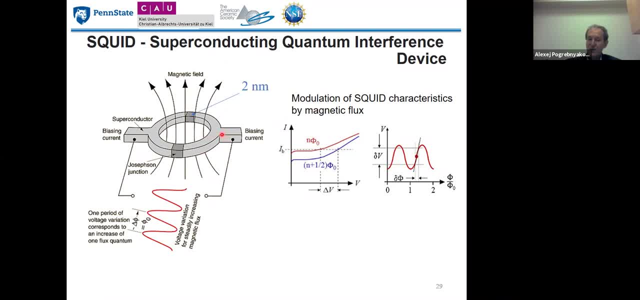 In the absence of external magnetic field, the system will be: these currents will be equal. But if you apply external magnetic field that will penetrate through this ring, it will induce a circular that will be added to this current that is passing through it. 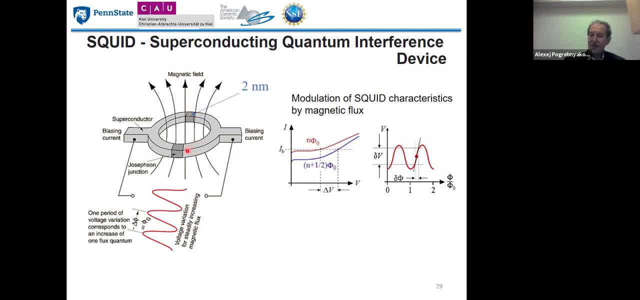 And it will change the current through each of Josephson junctions And this way we can modulate the current through the all the voltage. If you apply constant bias and current, then application of external total current, turning off external magnetic field. 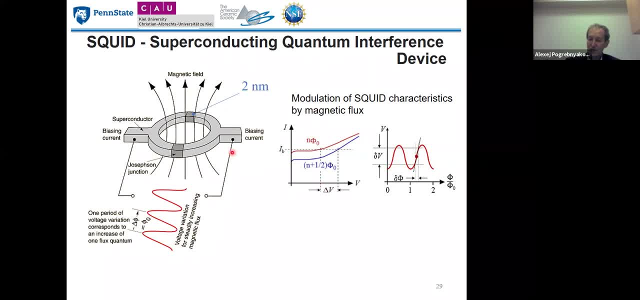 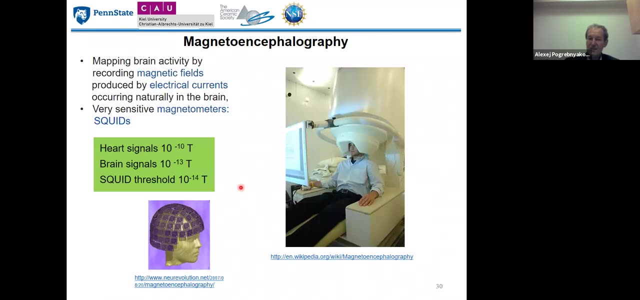 will change the voltage. voltage drop on this structure. This is a basis of magnetometry measurements of extremely high sensitive magnetometers, which is used, for example, in magnetoencephalography. Magnetic signals of brain can be measured using magnetometers. this squid arrays because the threshold of sensitivity for squids is near the quantum limit, about two times above the quantum limit. 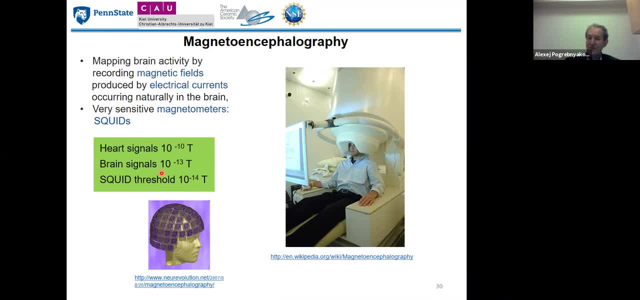 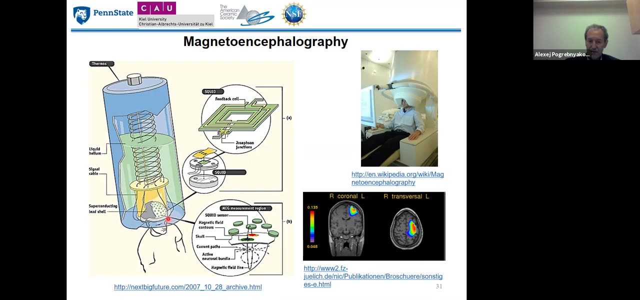 So the brain signals are much stronger than the sensitivity. so these magnetometers are currently used And what we can see here is just a cartoon that's showing that this array of magnetometers are conducted to electronics And we can see the brain activity in vivo. 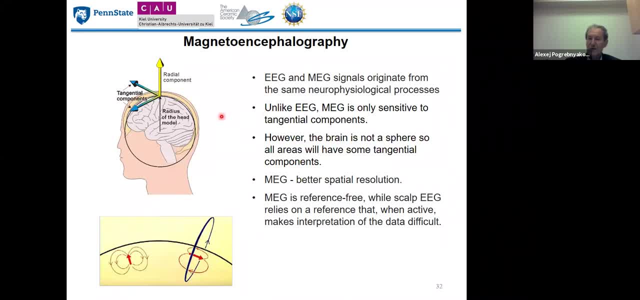 So magnetic signals from the brain are much smaller than electric signals. So electroencephalography measures much stronger signals than magnetic encephalography. But magnetic encephalography has many advantages. It has much higher spatial resolution. So one can carry out these studies before the surgery to find the areas where the surgery should be done, areas of pathology in the brain where the surgery should be conducted. 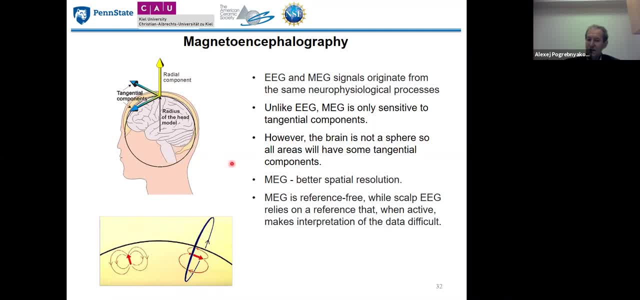 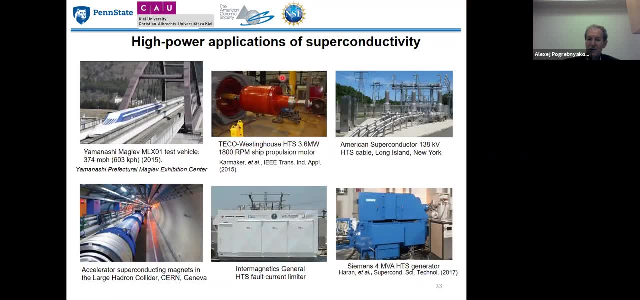 But in general these two methods complement each other, Thank you. And the other applications of superconductivity include high power applications where this levitation of magnets is used, So well-known bullet trains or maglev trains. magnetic levitation uses superconducting cables. 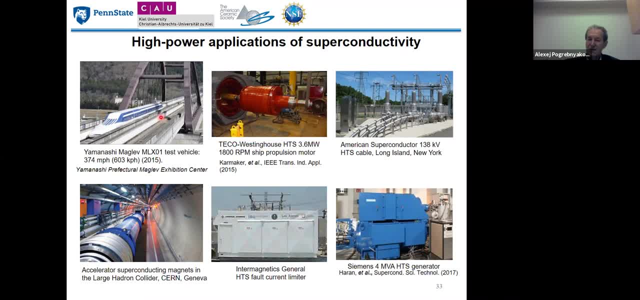 And magnetic constant magnets that allow the train to be floated over the conduction path. Also this superconducting magnets produce propulsion of the train. Also, the superconducting cables are used in motors for transmission. High, very high density, Density electric currents. 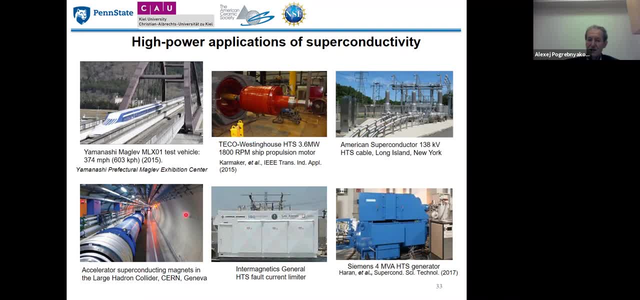 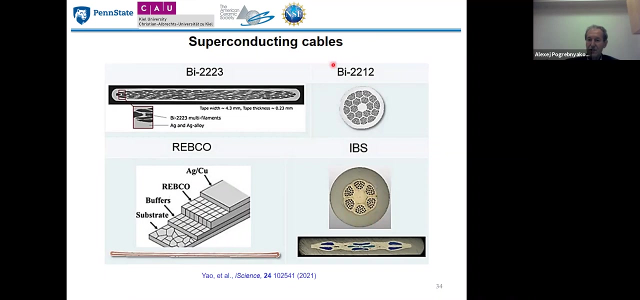 And they're used in CERN in particle accelerators, in particle for focusing the particles, for bending the particle beam, And in, for example, Zeman's makes, high temperature superconducting generators, Superconducting cables of high made of high temperature superconductors can be made out of round wires or after rolling from tapes. 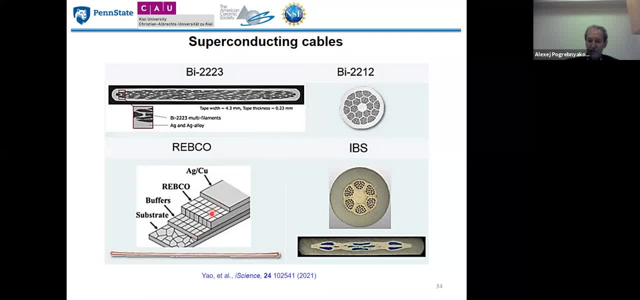 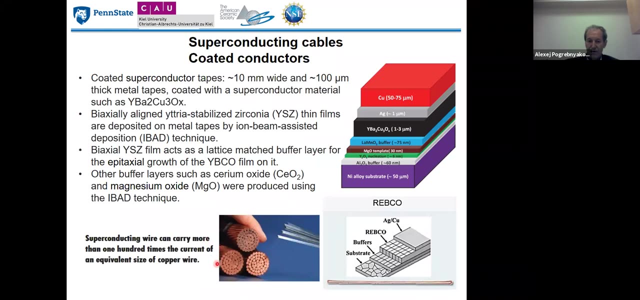 And here we see the cartoons showing the so-called second generation tape of superconductors, And. And Superconducting wires can carry more than 100 times higher current density than equivalent copper wires, But they, because these are again, these are ceramic materials. they require. 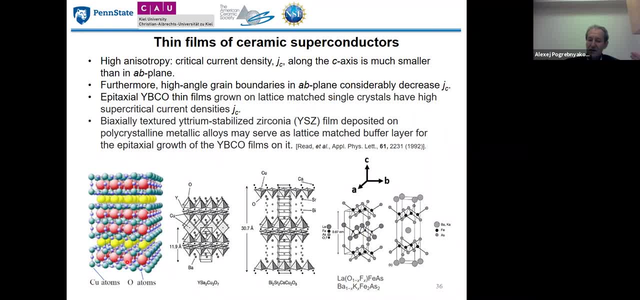 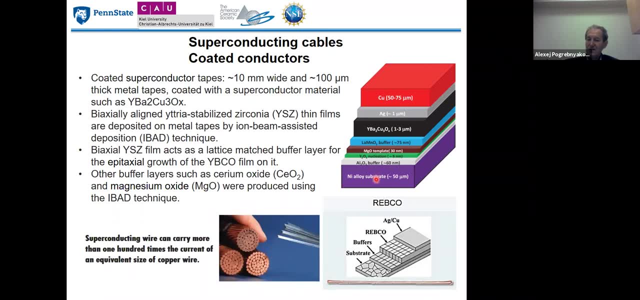 They require some Texture. One cannot deposit high-temperature superconductors directly on flexible metallic substrate. One has to deposit first buffers, or maybe multiple buffers, on top of which you can epitaxially grow a layer of high-temperature superconductors. 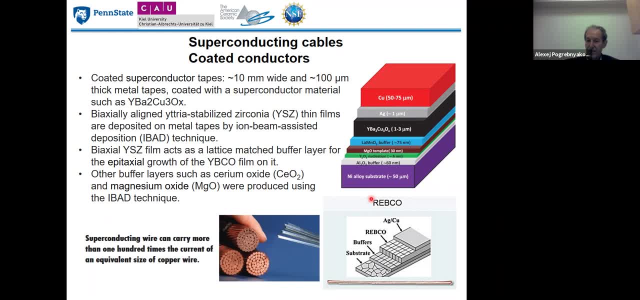 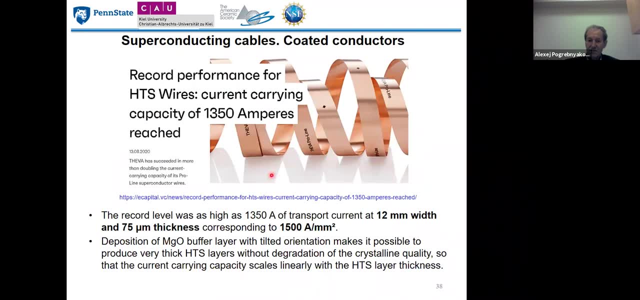 That is, the of a superconducting cable, And this is the latest achievement in the production of high temperature superconducting wires and tapes at the company of Teva, The last year they have achieved the record of 1,500 amperes per square millimeter. 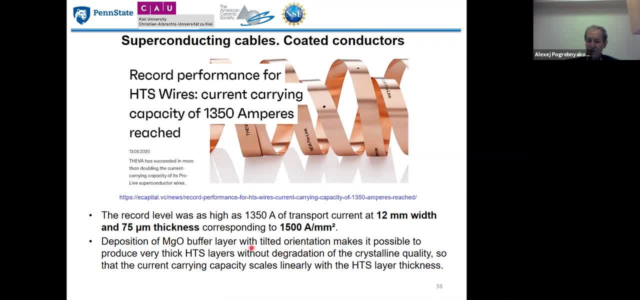 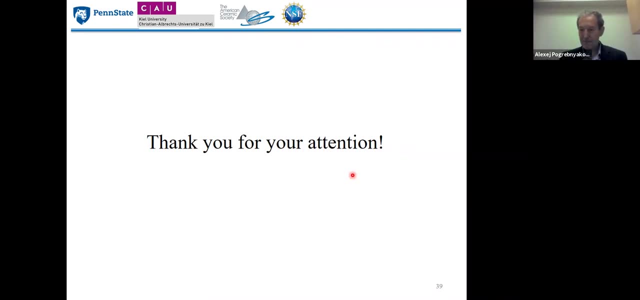 critical current density. Because of this, they found how to improve the process of fabrication. So thank you for your attention. All right, Thanks so much, Alexey, for this great talk. I know we have only a couple of minutes for questions. 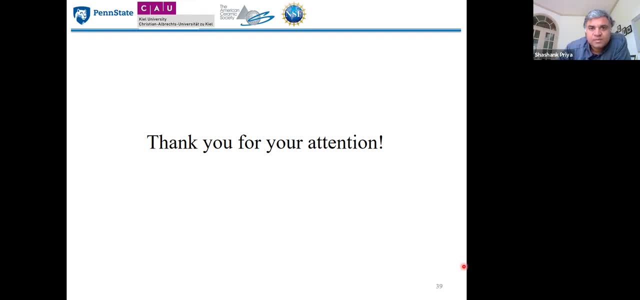 It'll be great if you have some for Alexey. Actually, I'm very impressed. Every time I hear about superconductors, you learn something new. It's such a complex physics and such exotic phenomenon, But one of the things which I would love to explore more. 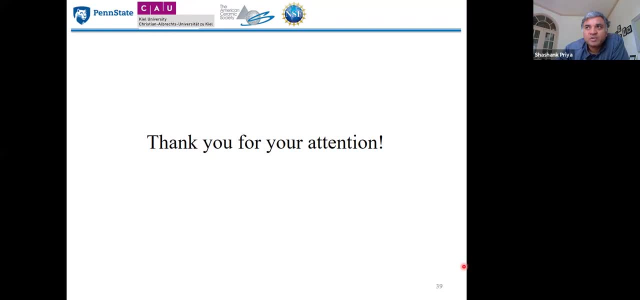 Alexey, is these magnetic measurements. So the best we all know we use VSM machines and some people use the squid magnetometers for measuring the magnetic material properties And the squids can go down to, I guess go down to almost like a picot-tesla level. 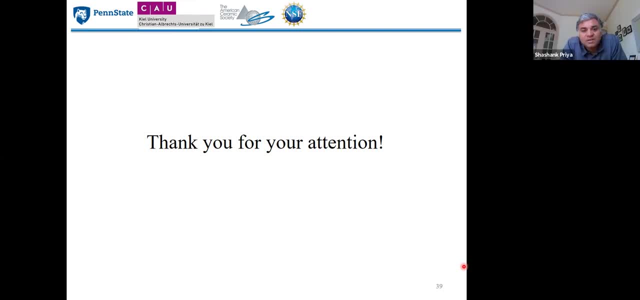 measurement in an isolated room. So for us as as a magnetic material researchers, we are always trying Воылand to study an eternity tolerance, times limit, to find a way to just push that measurement limits right. and and same thing in biology, like the brain signals, especially the neuron firing, is on the order of like 0.1 or 0.01 pico. 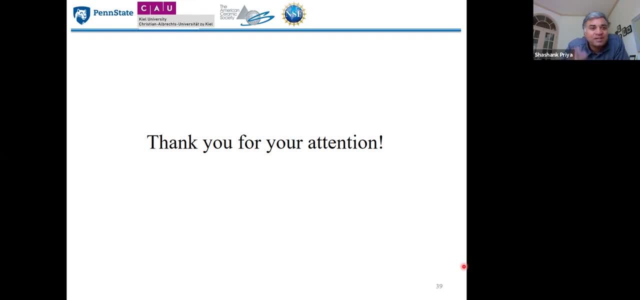 tesla level. yes, yes, um. and if we can, yeah. if we can, for example, make a superconducting helmet and it can start to measure the brain signals, like a non-contact, non-invasive, that'll be great. but it just requires huge amount of magnetic bias like several teslas. 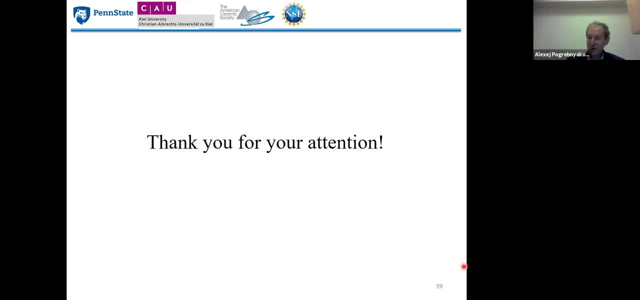 and that's a challenge. yes, this is a fascinating. properties of superconducting quantum devices. yes, that's how superconductivity is used. yeah, so to both these: measurement of magnetic materials and measurement of brain signals. yeah, i'll be. i think super conductors are these state of the art in both cases. 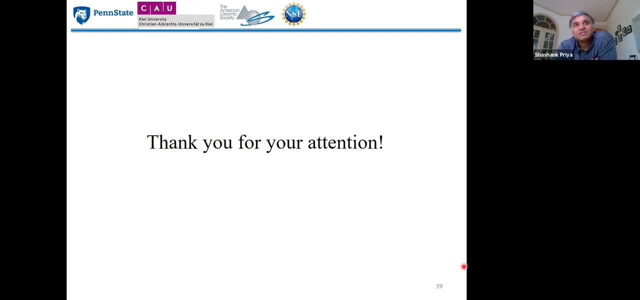 but the only challenge is that it requires low temperature and and it requires a huge amount of bias fields, um and and so. so any way to reduce both these things- and i guess this is the holy grail here- high temperature, and that is my high temperature superconductor. 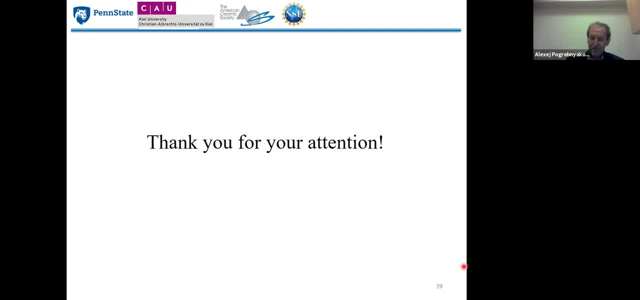 are widely investigated and so many efforts were put into these tiles to create this superconducting wires made of high temperature superconductors because, for example, in CERN, this latest experiments, they put in very traditional metallic niobium-titanium wires that developed. 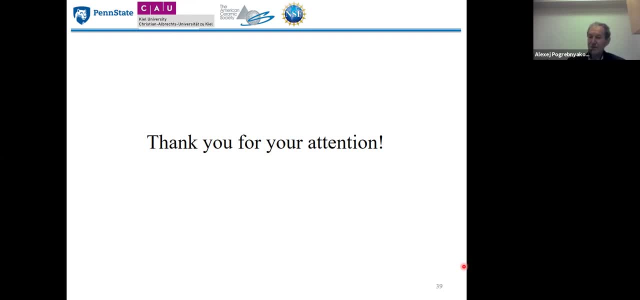 the process, the technology of production of these wires were developed in the 50s, In the 1950s. they still use this, although just last year General Electric's produced more than 1,000 of these. They still use this, although just last year General Electric's produced more than 1,000 of these. produced more than 1,000 of these. They still use this, although just last year, General Electric's produced more than 1,000 of these. They still use this, although just last year, General Electric's produced more than 1,000 of these. 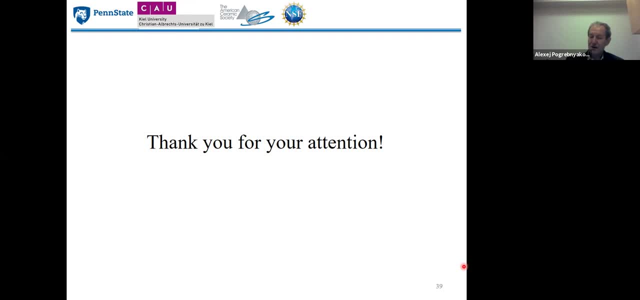 These were magnets for the CERN that were made from niobium-3 tin that has about twice the temperature of niobium-titanium alloy, and that allowed to make these magnets smaller and give these large physical chambers, which are the detector chambers, more space for. 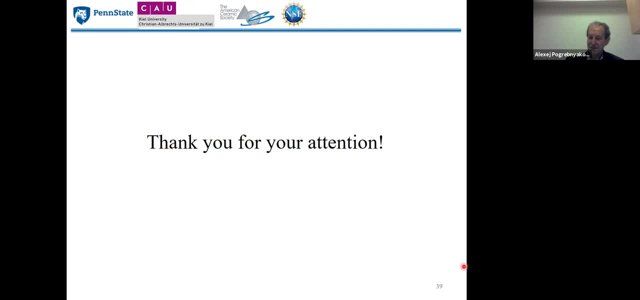 which are the detector chambers, more space for, for upgrading these experiments? Yeah, that's excellent. This is just an amazing topic and continues to remain very widely investigated topic. I have a quick question. Yes, Sanjay. So on the note of a high TC superconductivity, which is actively pursued, as you're pointing out, around two years ago or one and a half year ago in 2019, I came across some work on where they achieved the superconductivity at room temperature. I mean like 250k and 320k or something like that on lanthanum hydrides, however at very high pressure. So I think 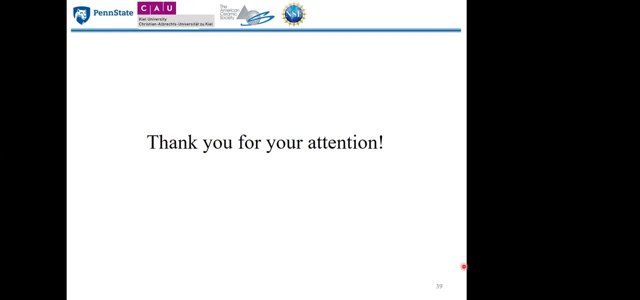 they are lanthanum-based and yttrium hydride-based systems. So do you get any comment on that? What's going on over there? Yes, you're right. A long time ago, Professor Mermin suggested that hydrogen, if it were condensed and made metallic, could be. 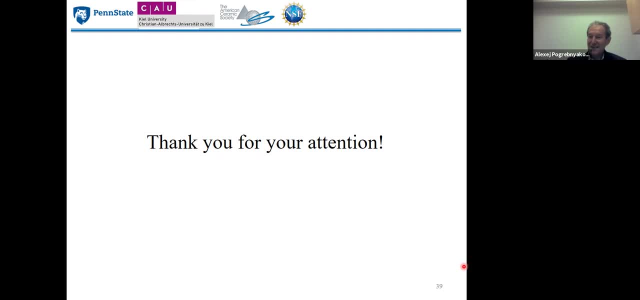 high temperature superconductor. However, this condensing, making the hydrogen metallic, would require some enormous pressures. So these recent experiments that you mentioned, they succeeded from 60s of last century up to now. They improved this technology of producing high pressures And they found that several compounds 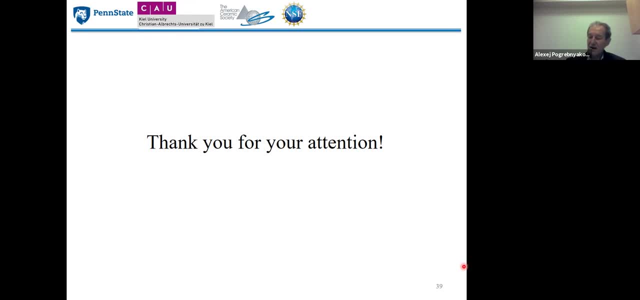 that contain lanthanides or a similar atom and like 10 atoms of hydrogen. So it's almost pure hydrogen, but it contains some. just pure hydrogen, but contains some can be. what they see is jumps in resistance at very high applied pressures. This experiments. 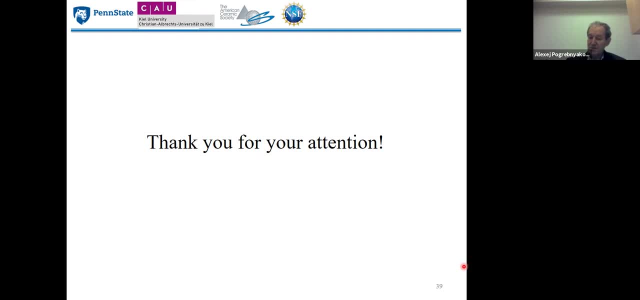 this: the volume of the samples is in tens of microns and they are non-uniform. So, although they already measure the structure and other properties, there were some objections that this were superconductors, superconducting, superconductivity brought about. 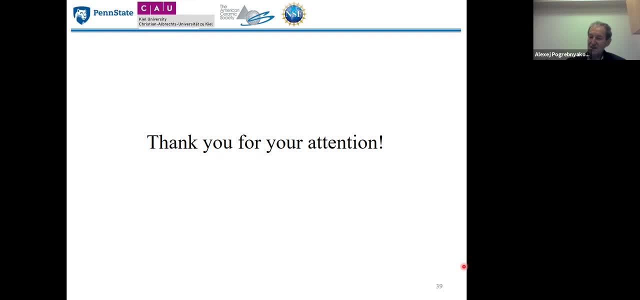 this drops in the resistance because just changing the crystal structure may drop the electrical resistance. So the teams that carry out this experiment strongly believe that they measure superconducting transitions, but there are some objections to that- And again, the level of pressures that are applied. 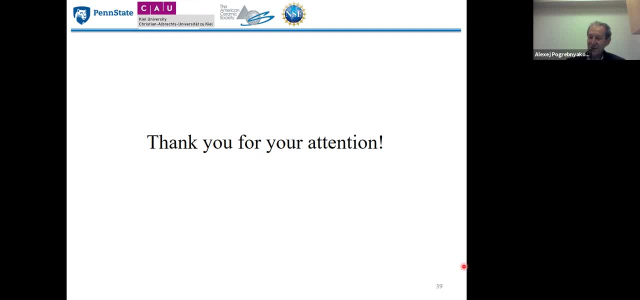 you know the Mariana Trench in the Pacific ocean, near Japan, near Japan, pressure at the bottom of this Mariana trench is about 1,500, more than 1,000 times smaller than the pressure that they apply at the laboratories.